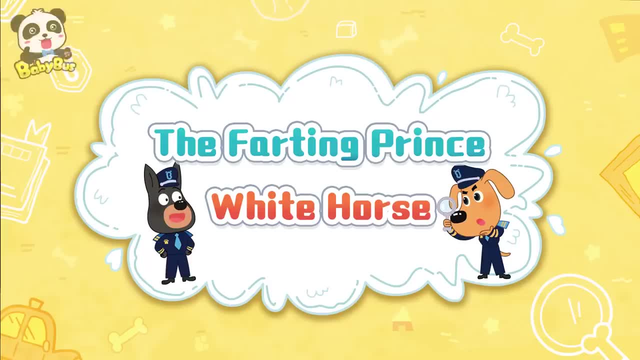 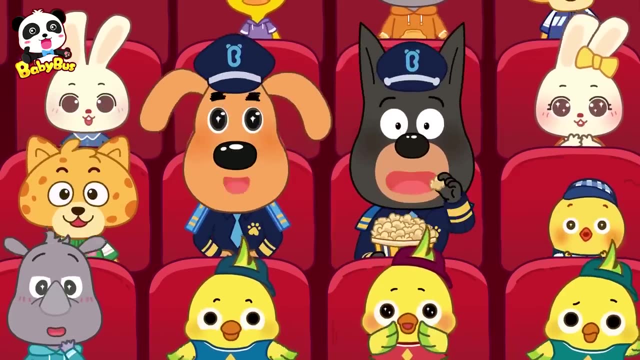 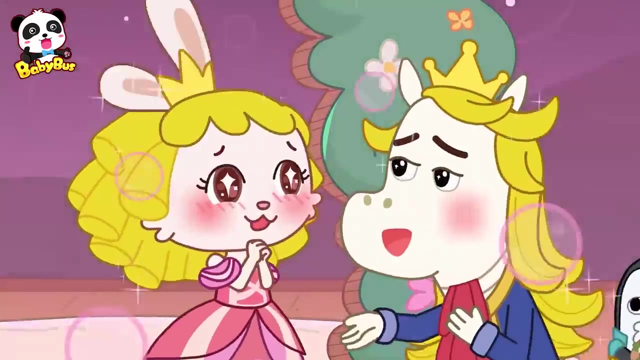 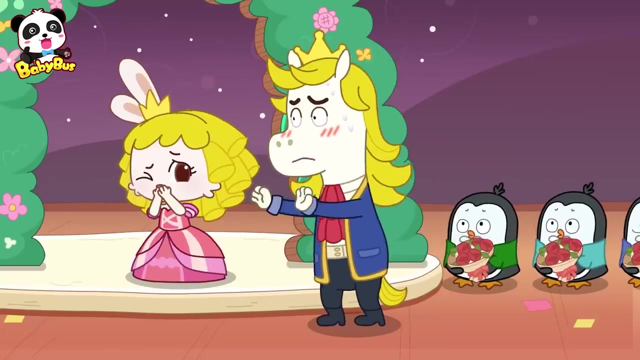 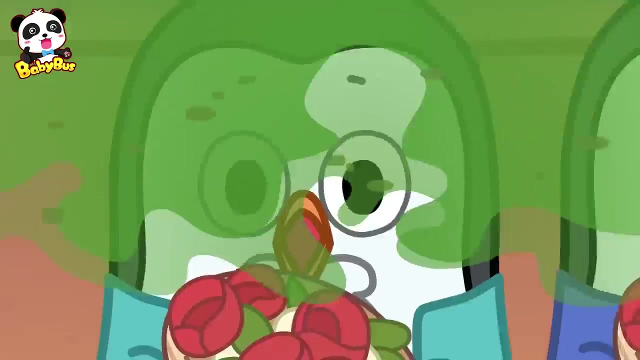 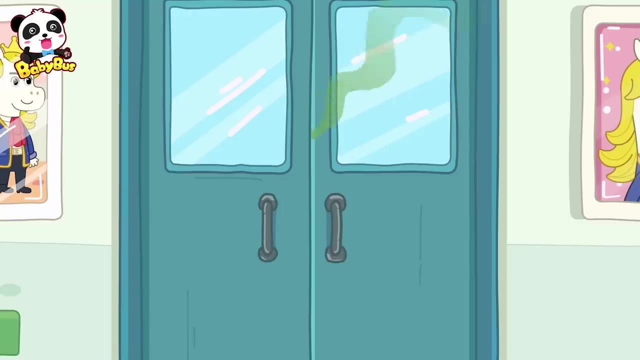 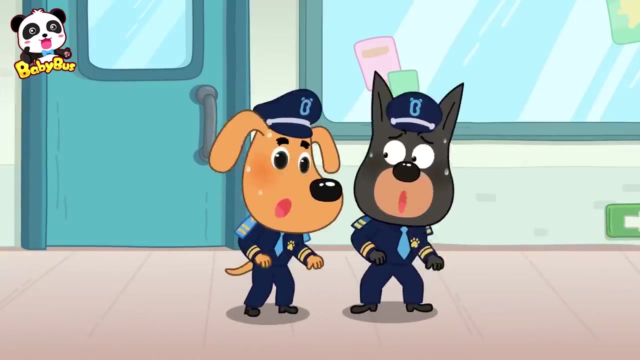 Baby Bus, The Farting Prince White Horse, My dear Snow White, will you marry me? Yes, I'm sorry, I didn't mean it, I just It stinks, It really stinks. Sheriff Labrador, Mr White Horse. 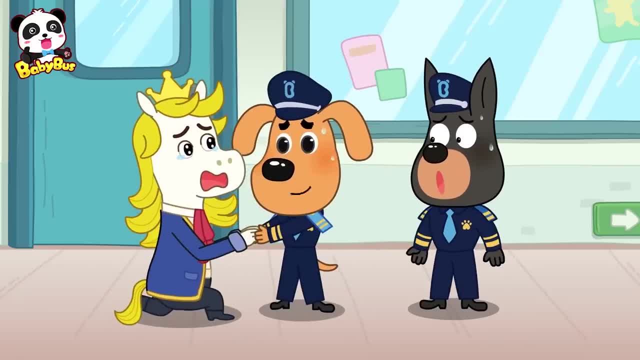 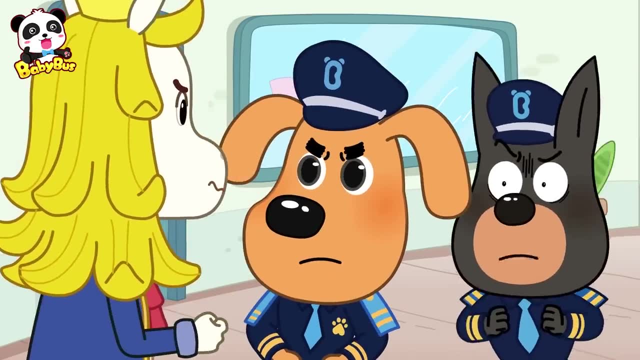 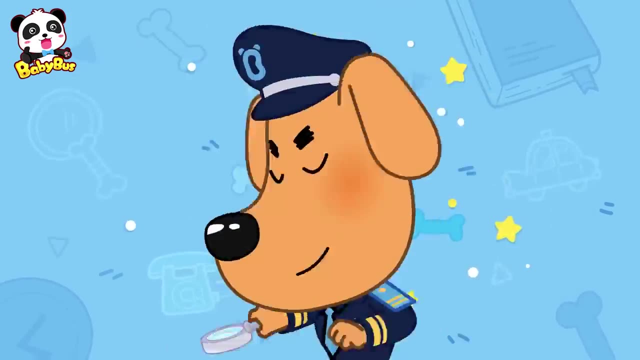 Help me. please Calm down, Mr White Horse. What's going on? Someone must have set me up. That's why I keep farting. What? Please find out who did this. Don't worry, There's no case that I can't solve. 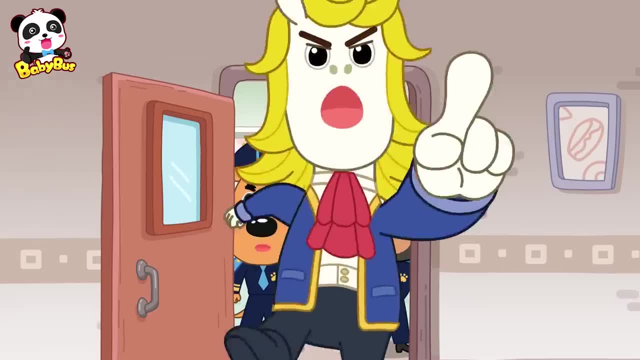 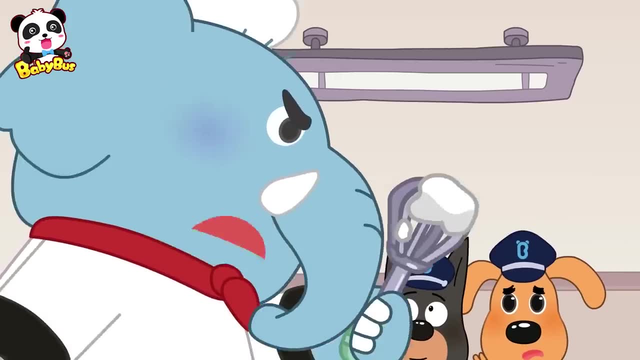 It was him who set me up, Chef Elephant. I was totally fine before I went on stage, but I had diarrhea after eating your cake. Are you blaming me for your diarrhea? I'm sure you have put something in my cake. That's the reason why I have diarrhea. 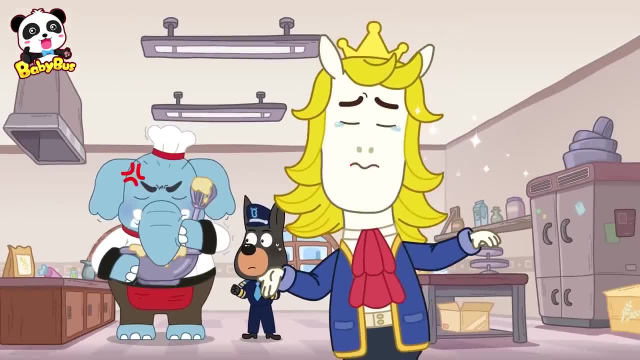 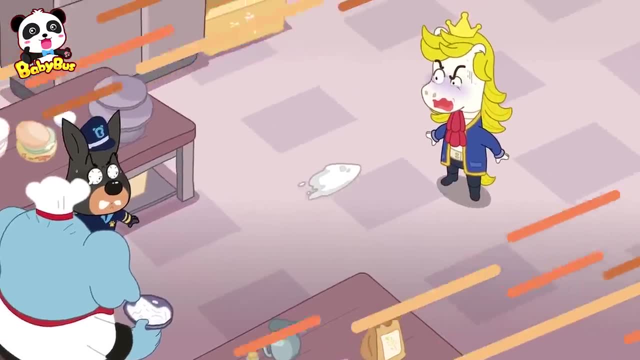 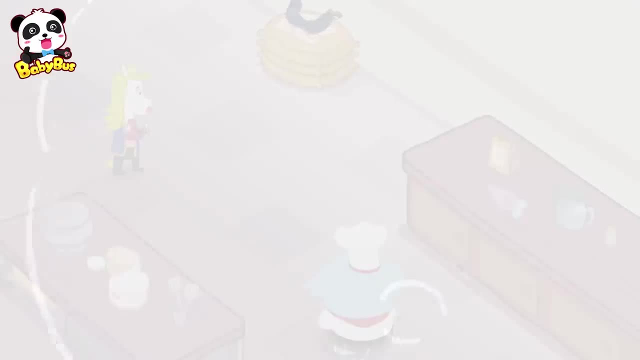 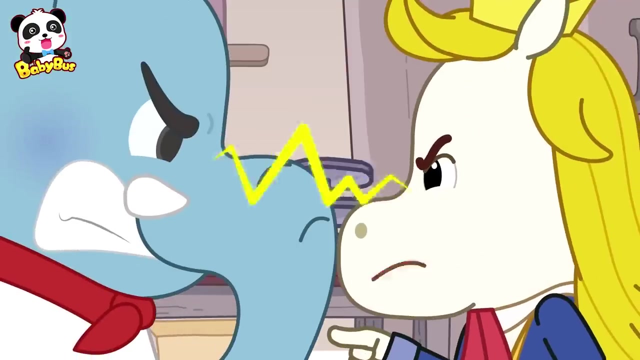 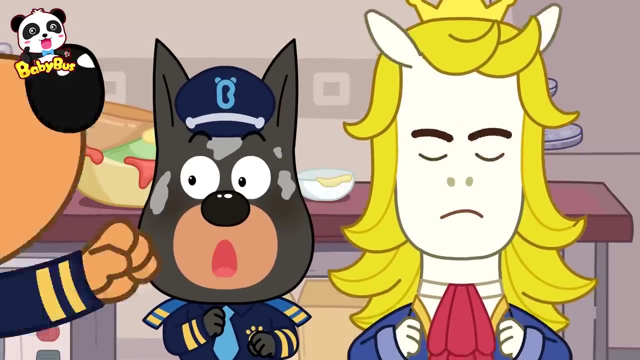 You must be jealous of my handsome face and that's why you have set me up. What are you talking about, Elephant? Are you trying to attack me? Please arrest him. Wait, It wasn't, Mr Elephant. What? Look at the plates over there. 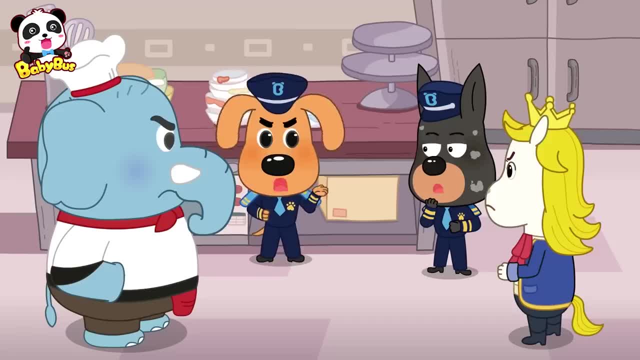 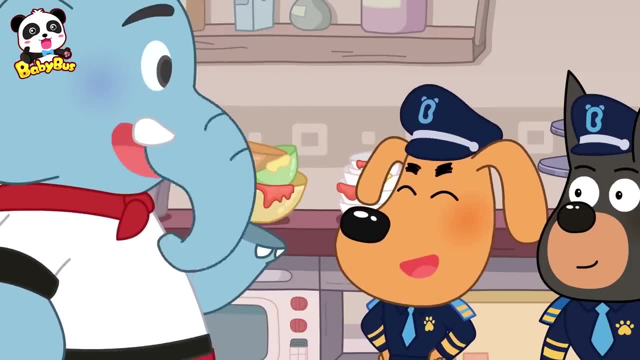 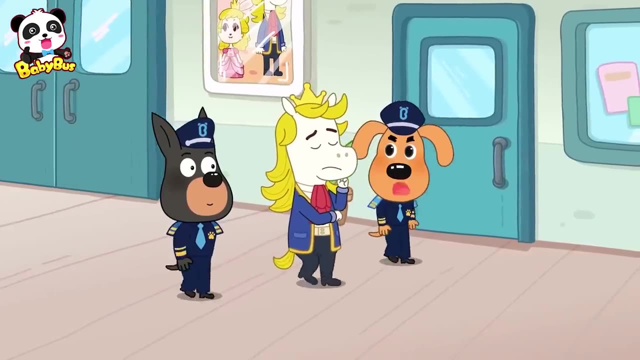 A lot of people ate the cake, but you're the only one who got diarrhea. That means there's nothing wrong with the cake. Exactly, Sheriff Labrador made a good point, didn't he? Well, Mr White Horse, what else did you eat before you went on stage? 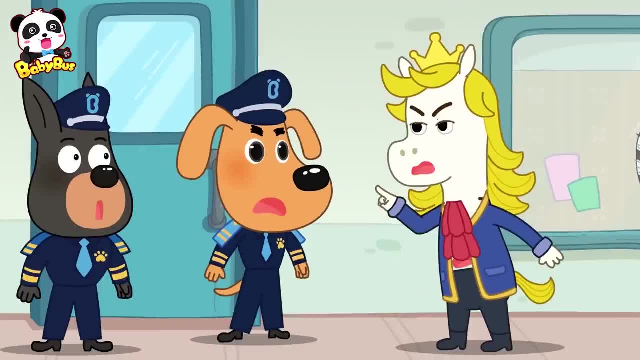 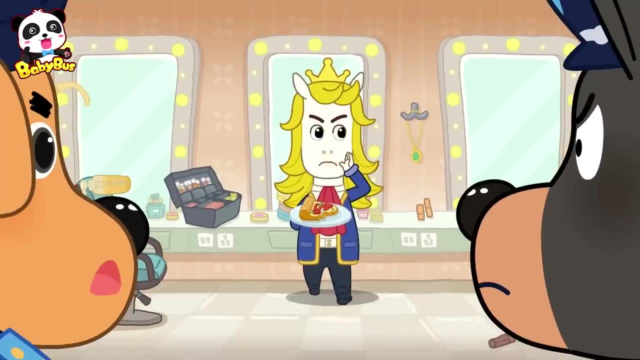 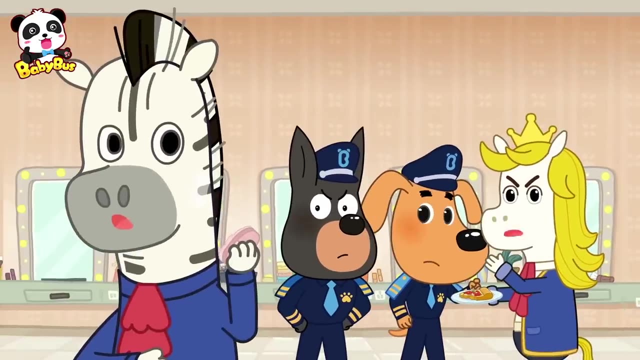 Oh, Zebra. Oh, I remember Found it. Mr Zebra gave me a slice of pizza. Look at this, Sheriff Labrador. I'm sure Mr Zebra has put something on my pizza because he wanted to replace me as the prince. 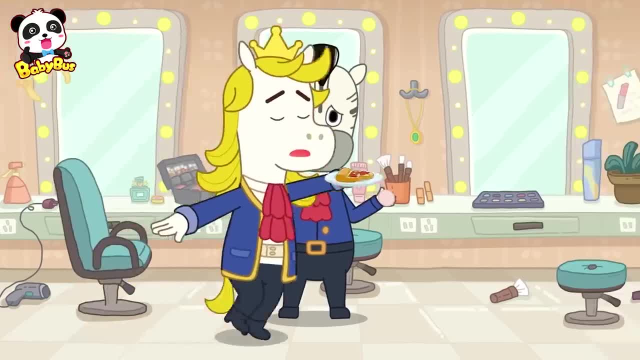 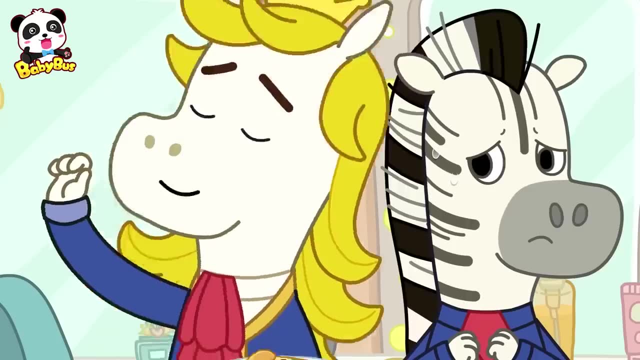 What? That's not true? Ha, You were jealous of me, weren't you? What? That's why you have put something on my pizza. If I am sick, then you get to play the prince. Oh, I didn't. 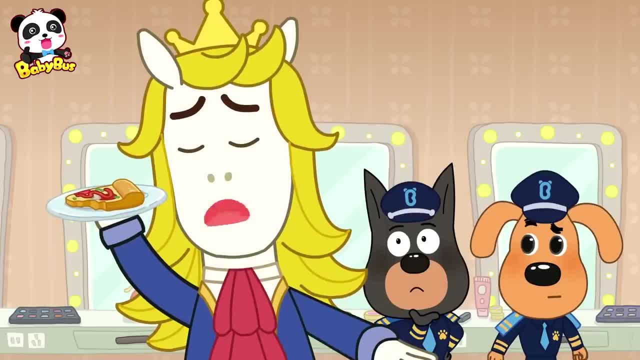 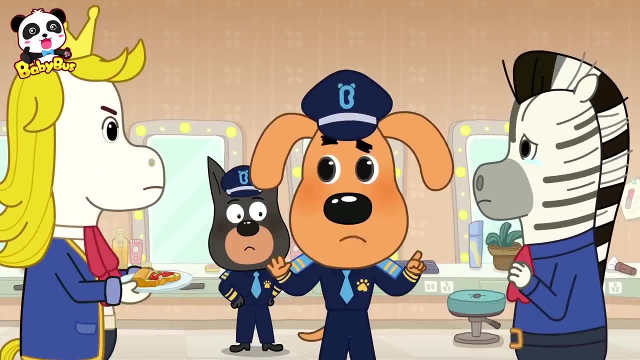 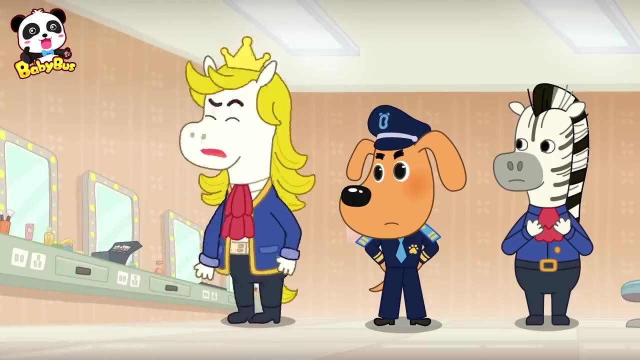 I was just born, this handsome. What's wrong with that? I didn't do it. Calm down both of you. We'll find out. if there's anything wrong with the pizza, Leave it to me. I can't hold it anymore. 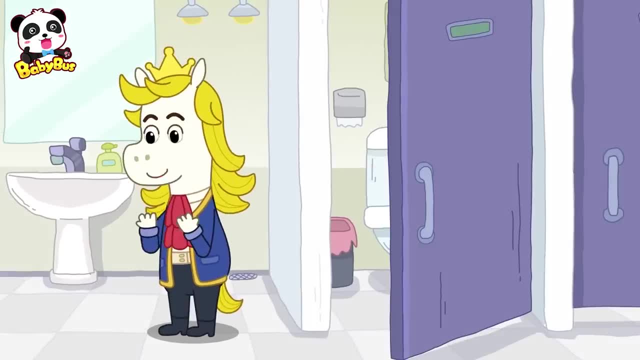 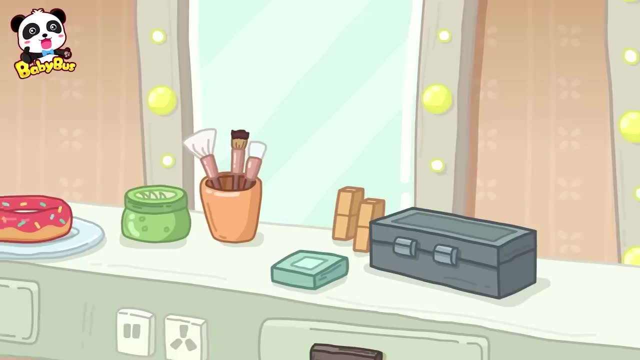 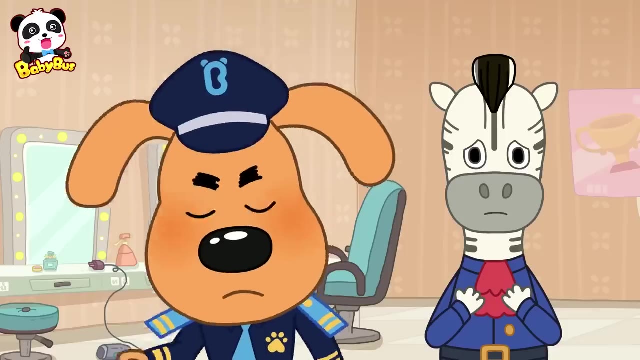 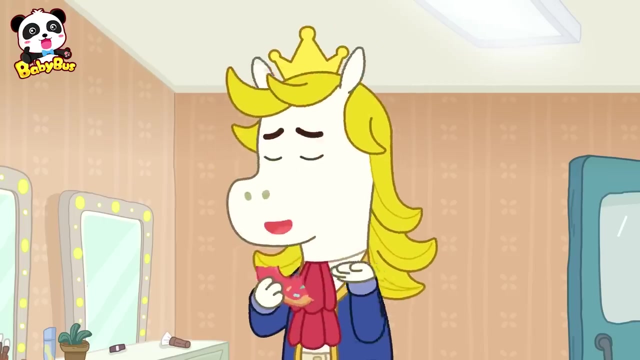 Oh, it's okay, I don't need to wash my hands. Oh, I'm so hungry. Oh, it's a donut. Mr White Horse, you should wash your hands before eating. Oh it's okay, Not a big deal. 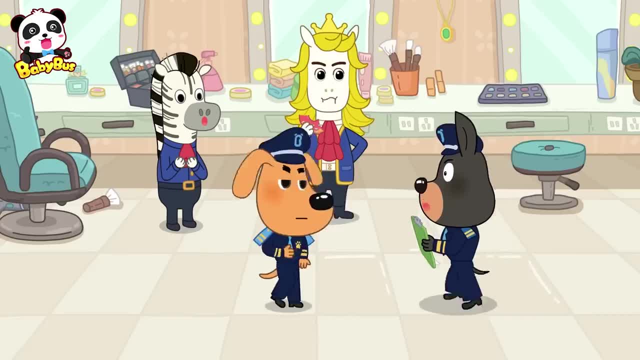 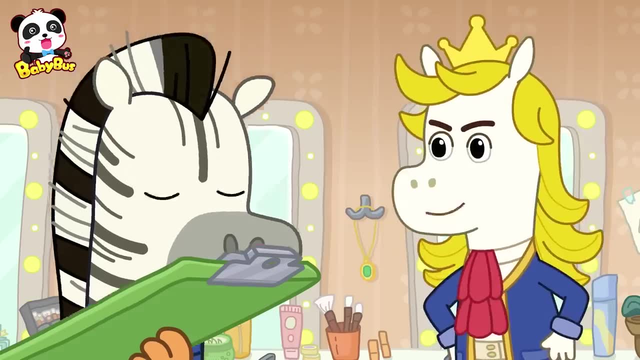 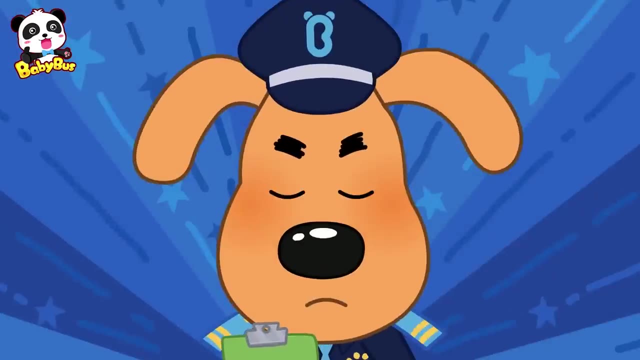 Oh, Oh Oh, Sheriff Labrador, a lot of harmful bacteria were found on the surface of the pizza. Zebra, it was you. It can't be. It wasn't Mr Zebra. The person who made you get diarrhea is yourself. 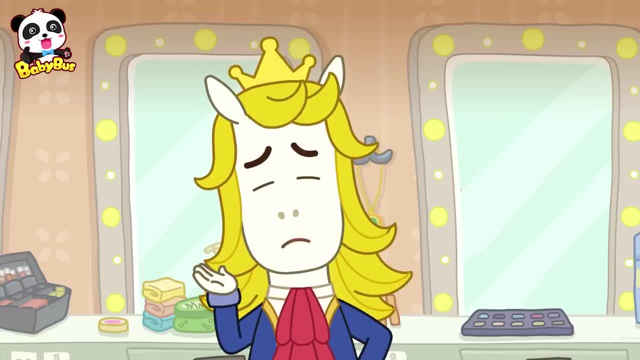 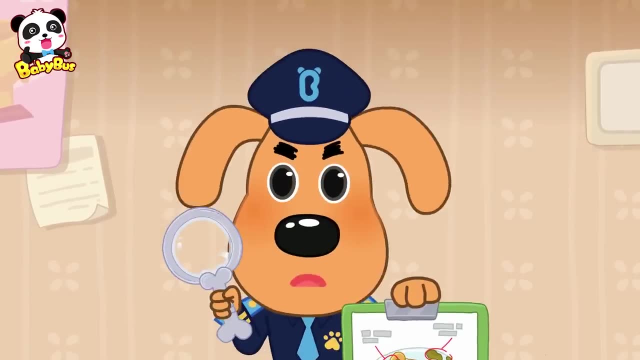 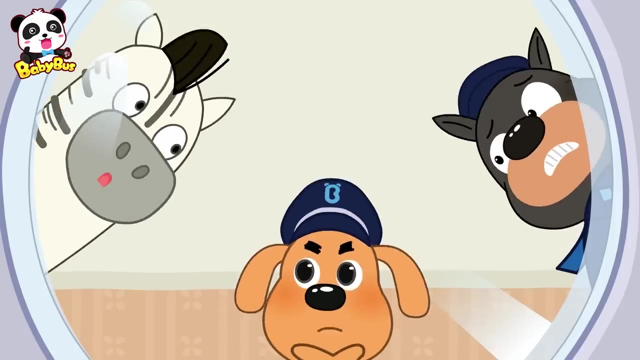 What Me? How can I possibly do that? According to the report, most of the harmful bacteria were found on areas where your fingers have touched. The bacteria were from your hands. Oh, Oh, You didn't wash your hands before eating the donut just now either. 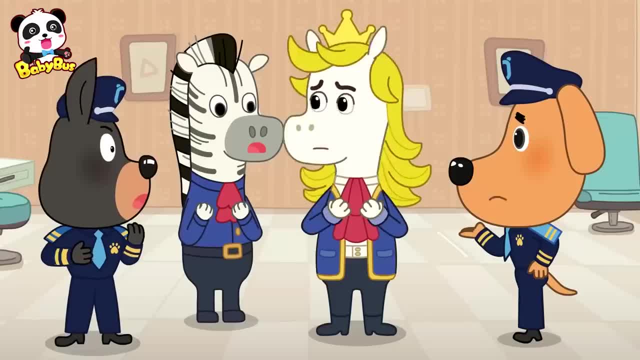 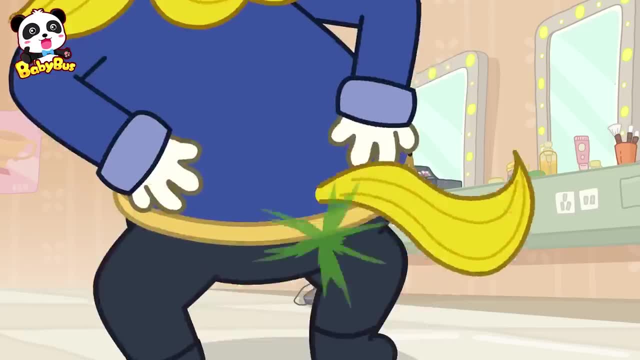 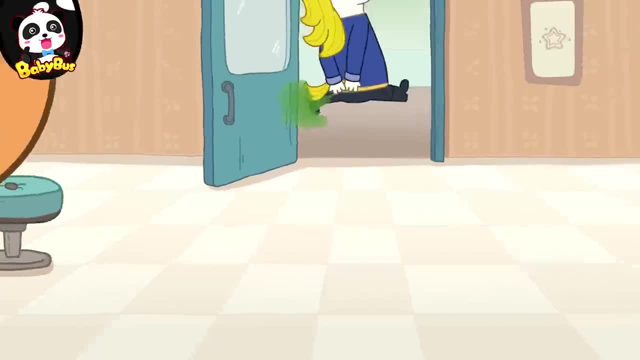 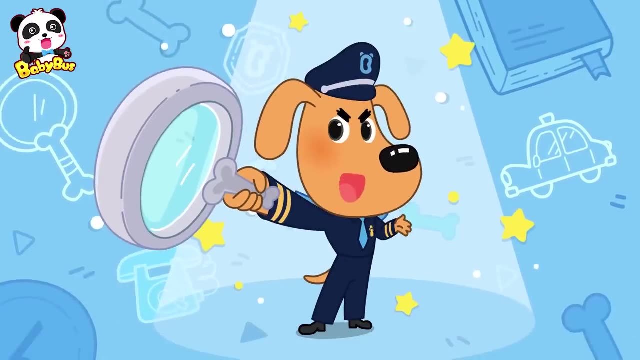 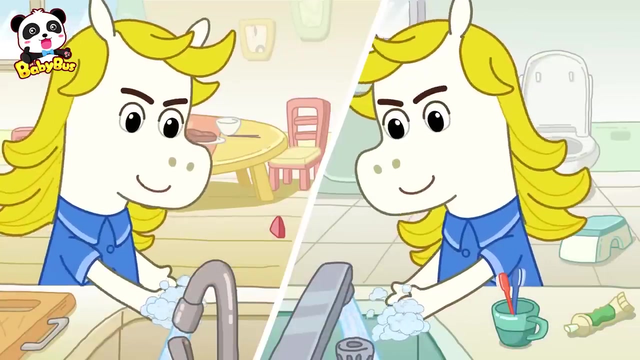 Oh, I'm washing my hands right now. I don't want to be the farting prince ever again. Oh, Oh, Oh, Oh, Oh, Sheriff Labrador's Safety Talk Kids, there are lots of bacteria on our hands. Wash your hands before eating, after going to the bathroom. 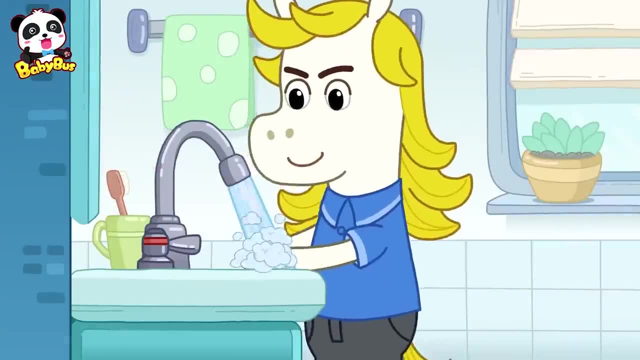 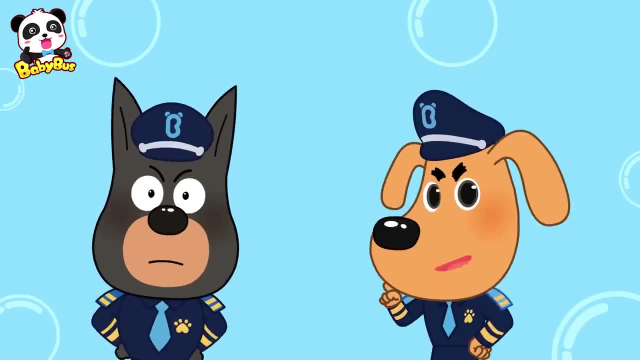 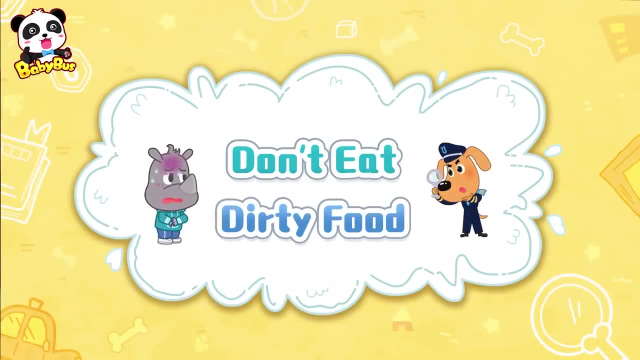 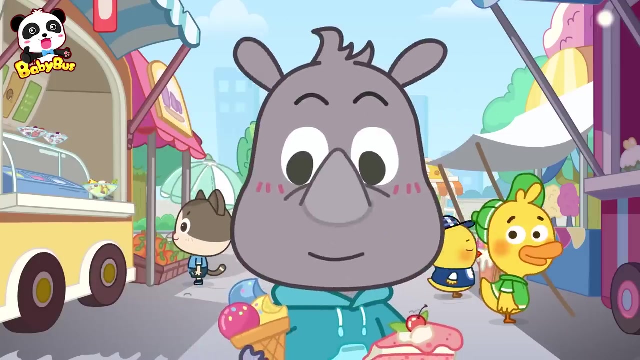 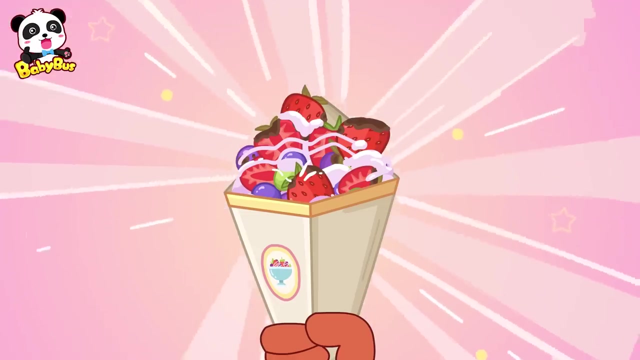 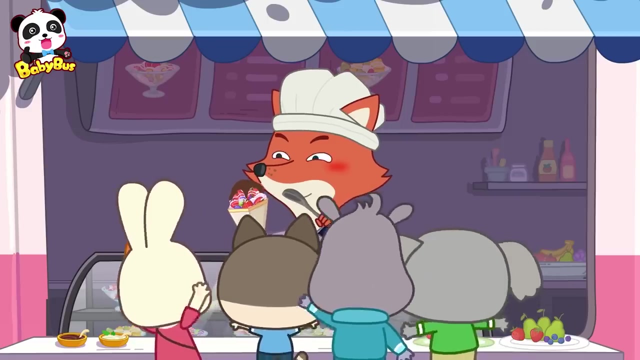 playing outside and using the public transit. If you don't, the bacteria can get inside your stomach and you can get sick. That's why we should regularly wash our hands. Don't eat dirty food, Mr Fox. I want one too. 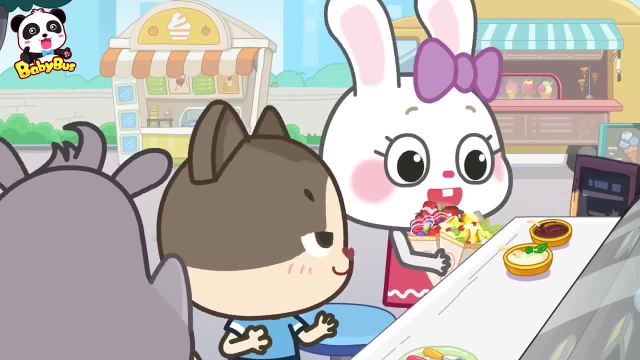 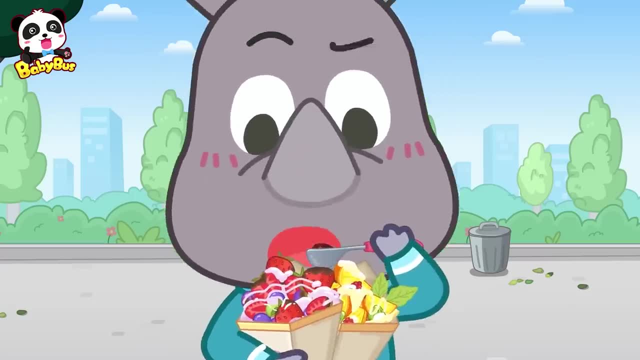 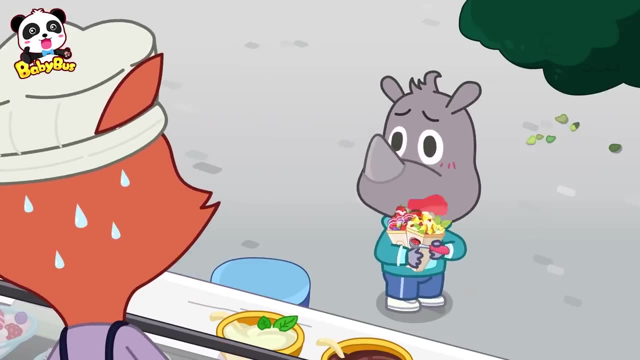 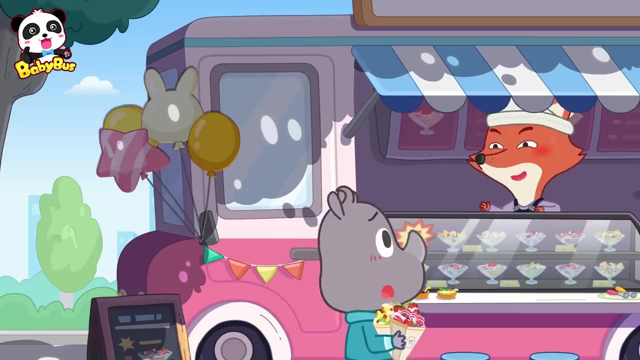 Alright, just a moment. Here, Here, Here, Here, Here you are. What's this, Mr Fox? what's this black thing? It's just chocolate. You seem to really like my salad. I'll give you another one. 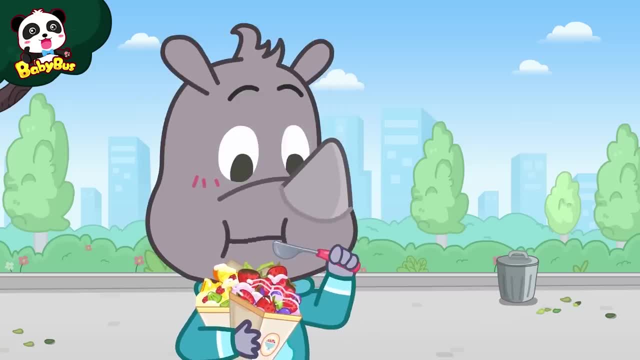 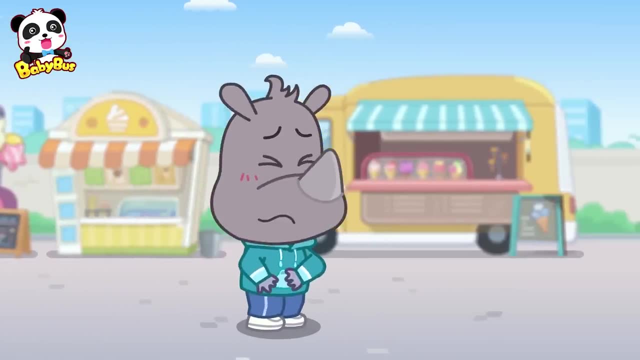 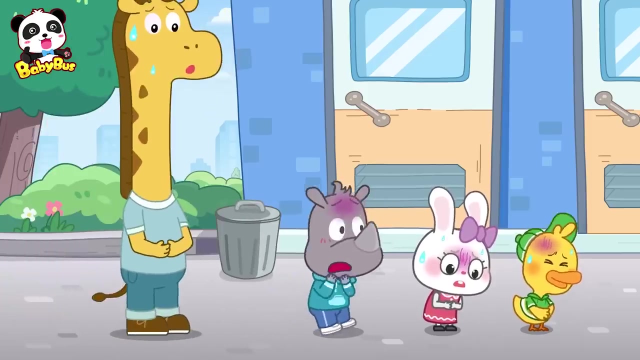 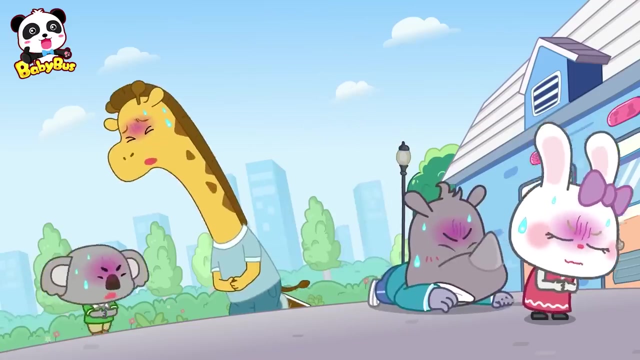 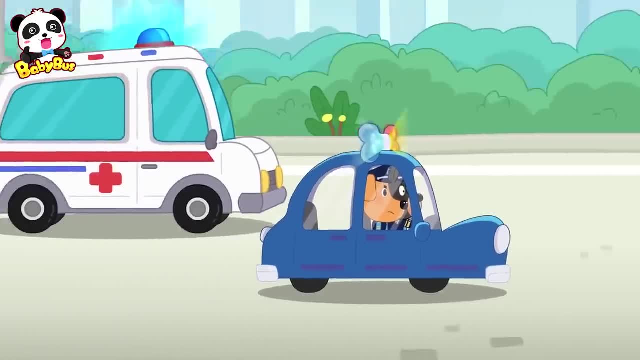 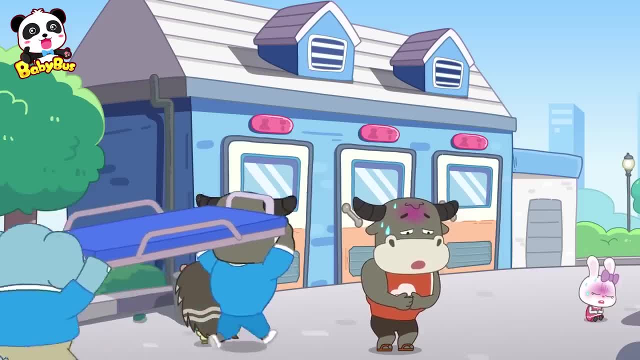 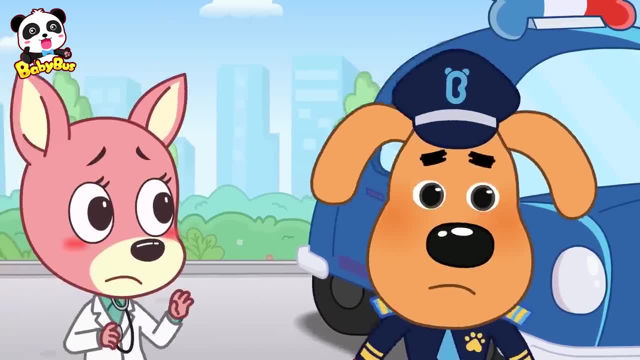 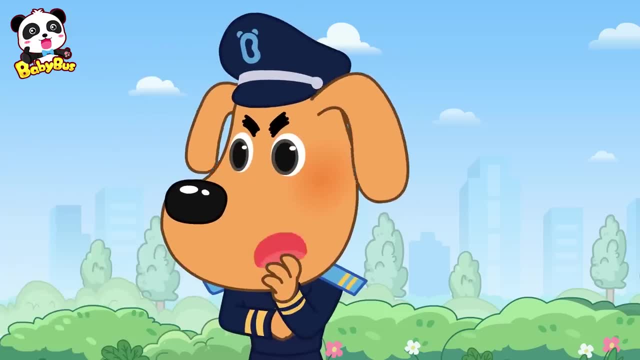 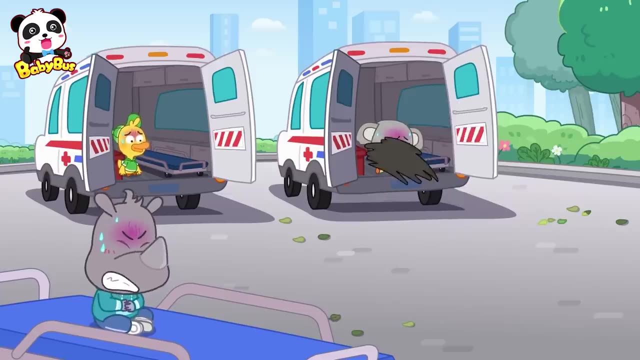 Oh my tummy, Oh my tummy. Oh, Sheriff Labrador, all these people got food poisoning. Huh, Something's wrong. Huh, Food poisoning, Gobi. please find out what they ate today. Hey kid, How are you feeling? 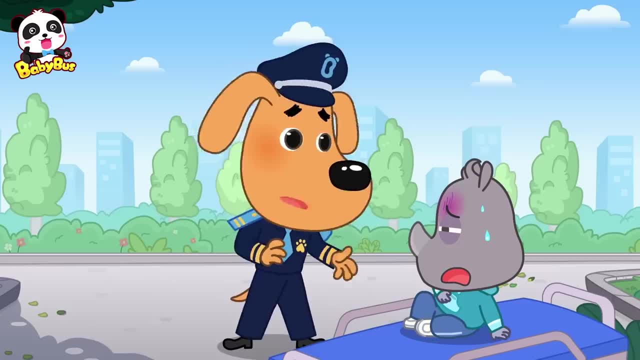 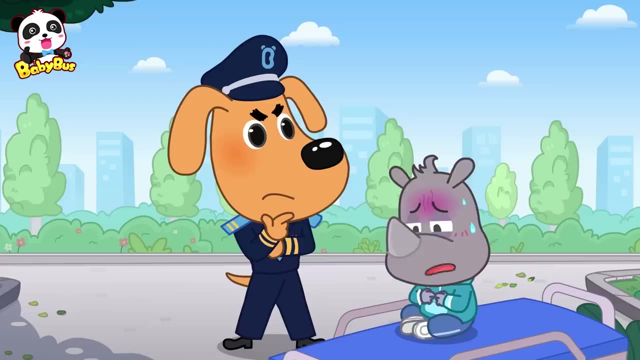 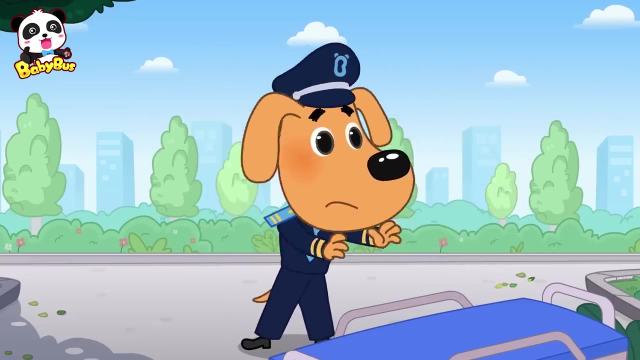 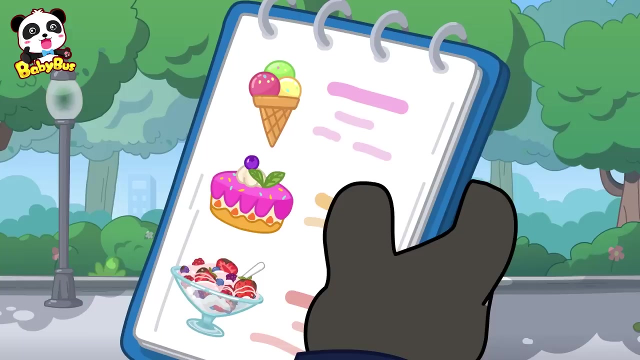 I've got the runs three times. Do you remember what you ate today? I had ice cream, fruit salad and a cake. Oh no, I need to go again, Sir. here's the report. They all had ice cream, cake and fruit salad. 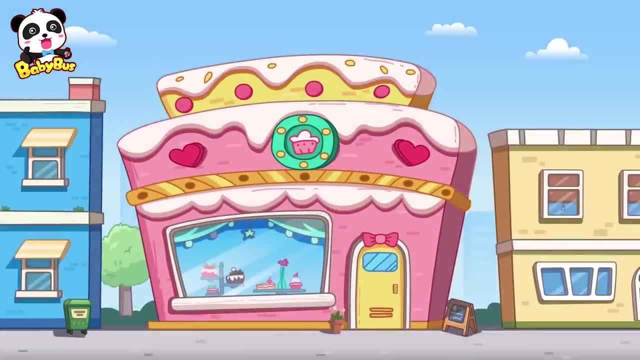 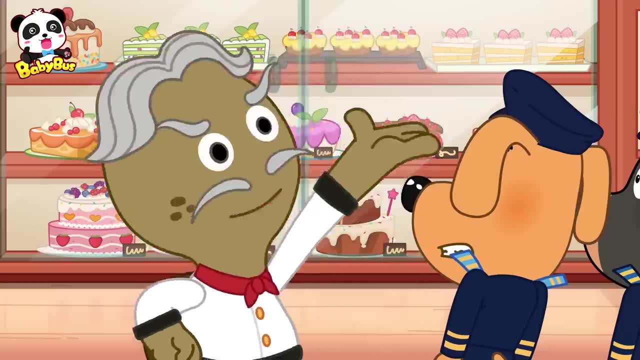 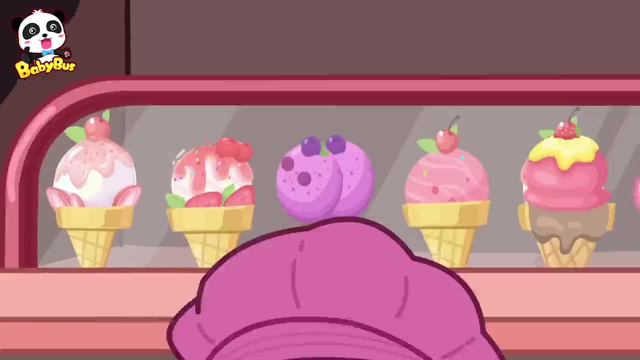 Let's go investigate these shops. It's not me. My cake shop has been here for 100 years. Such a thing has never happened since my grandfather's grandfather was here- Not me, I'm sure. I'm sure that nothing's wrong with my yummy ice cream. 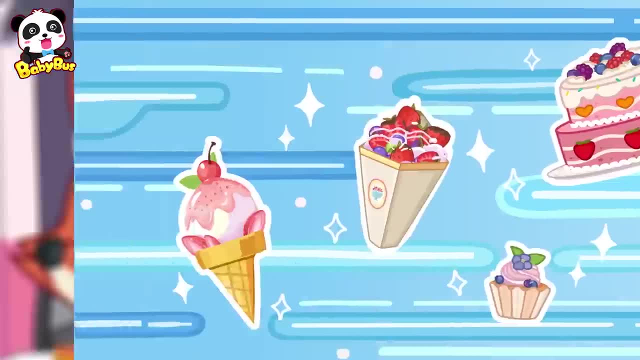 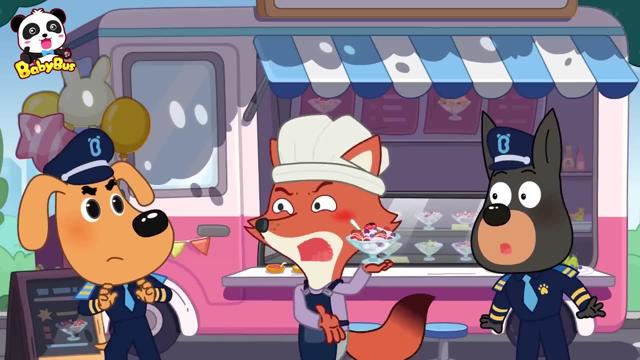 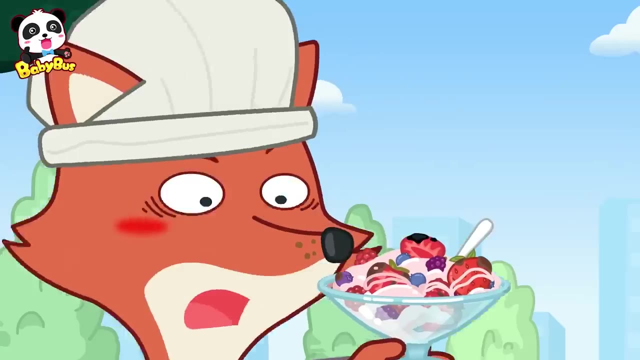 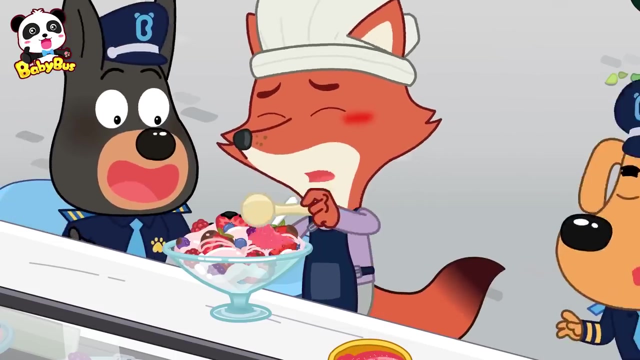 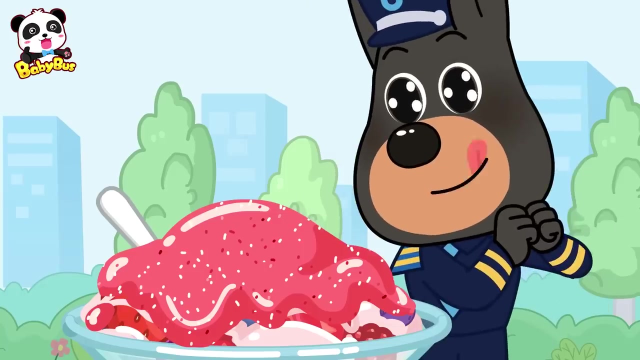 Look, My ice cream's fine. What Are you suspecting me? My shop is really clean. Every fruit salad is carefully selected by myself. I'm prepared by myself. Wow, I love fruit salad. I'd like to have one please. 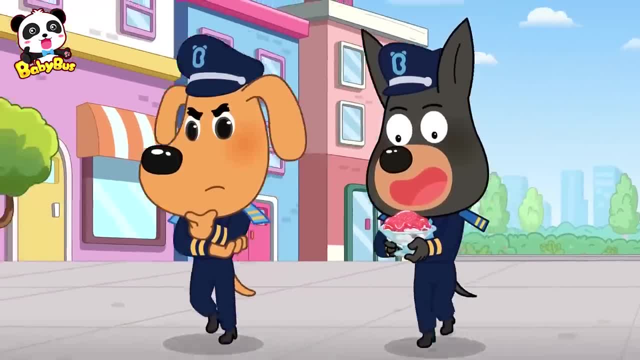 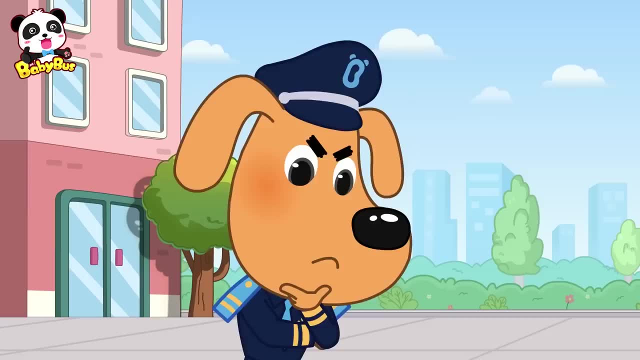 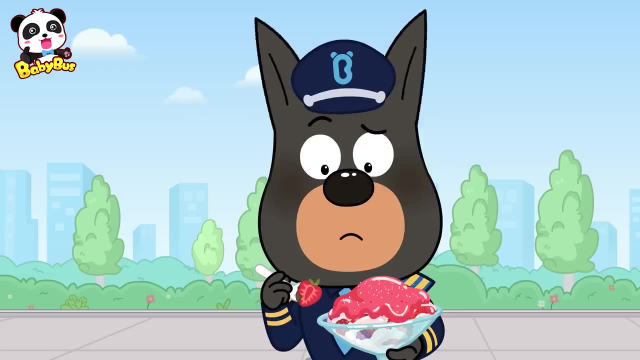 Great choice. I don't think there is any problem with those shops. Don't eat it. I smelled rotten fruit in Mr Fox's salad shop. He must be hiding something. What, What, Huh, Isn't that, Mr Fox? 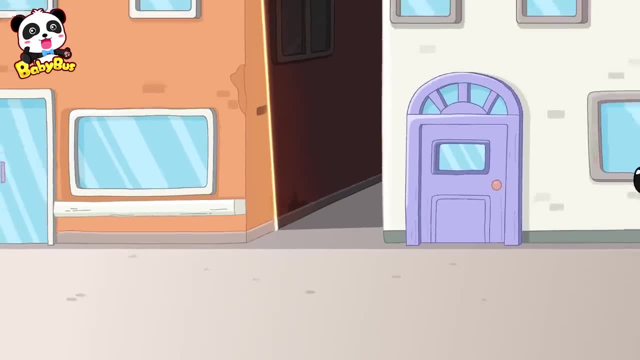 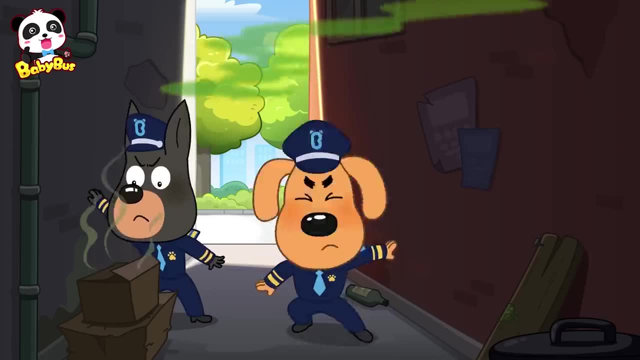 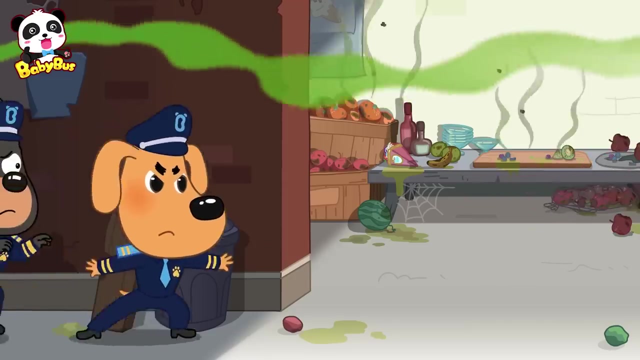 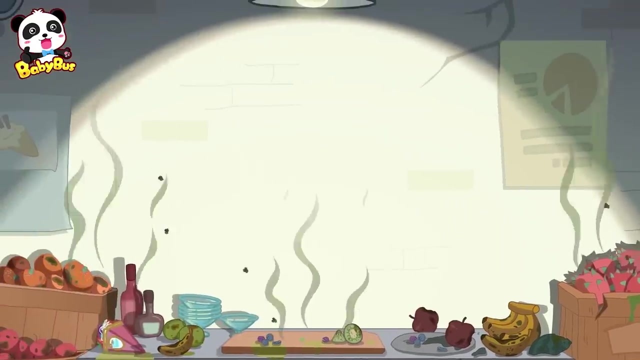 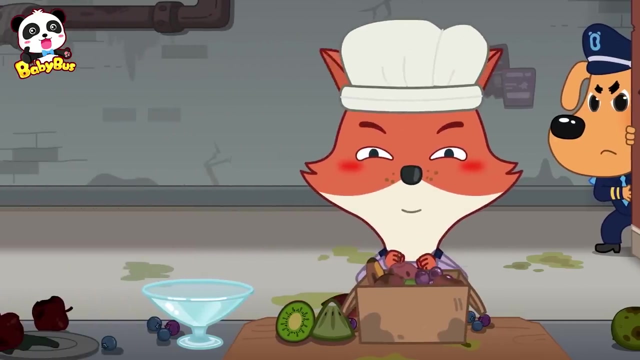 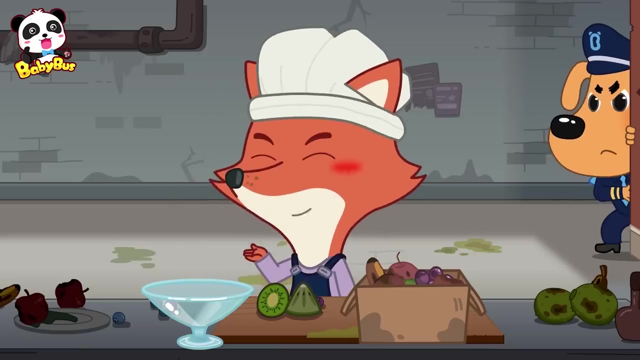 What is he doing there? Let's go follow him. Rotten fruit is everywhere Where Those police officers believed what I said. I don't care about rotten fruit, I'm not eating them. anyway. Mr Fox, It was you who made people sick. 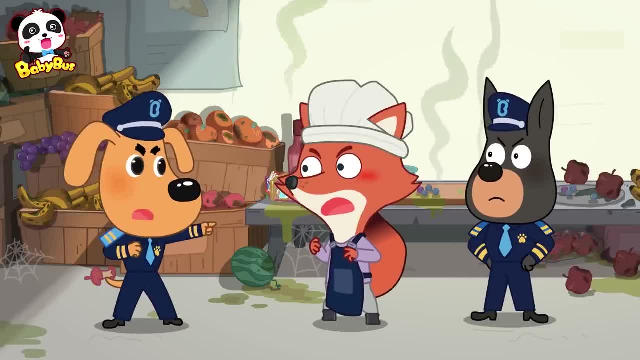 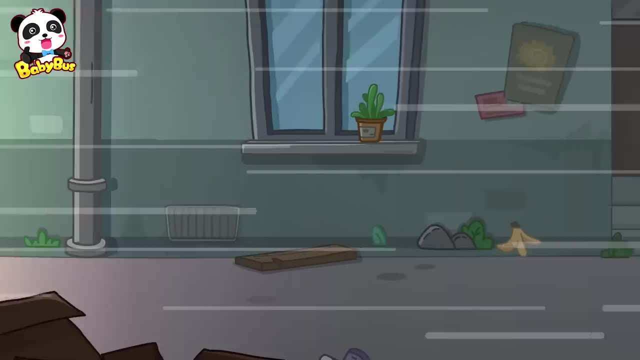 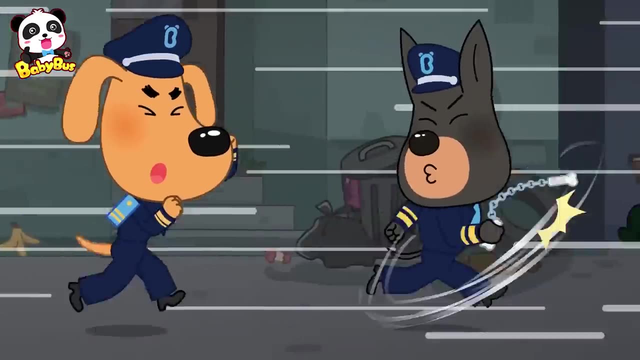 Police, Come with us to the police station. I'm gonna run, I have to. Let's go along with it. See you at the police station, We'll go back. Okay, Go along with it, I won't leave you. 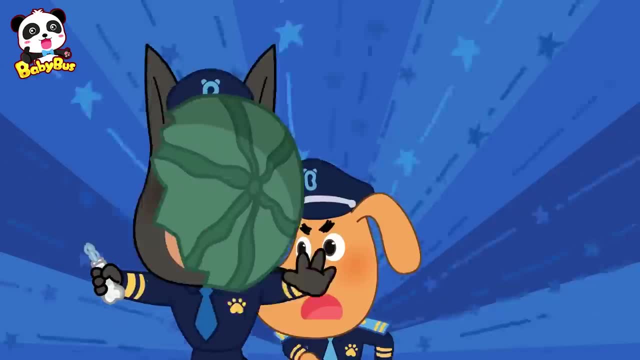 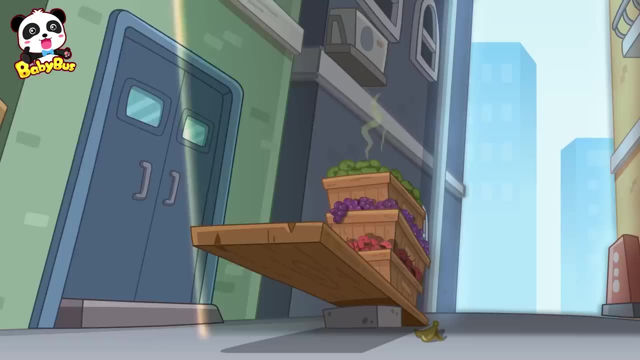 I won't This time. I will keep them coming. You're such a nobody You must run away. I'm going to hide into the forest. Okay, Let's go. They're coming. Yeah, Let's get out of here. 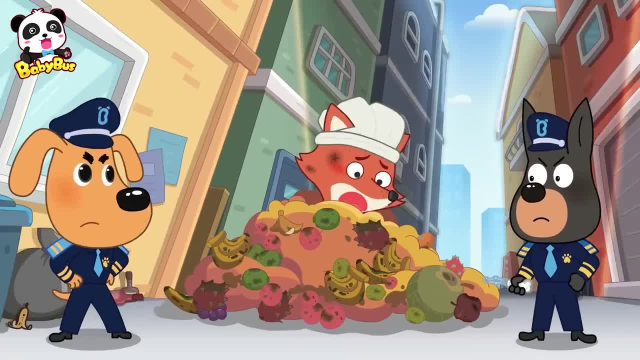 Spend some time here. I want to go home to Mr Fox. Go home. No, I'm going home, Let's go. Let's go. You're going to go home. I'm going home. No, You're going home. 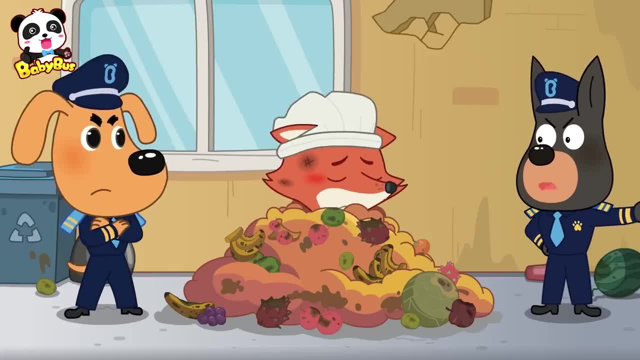 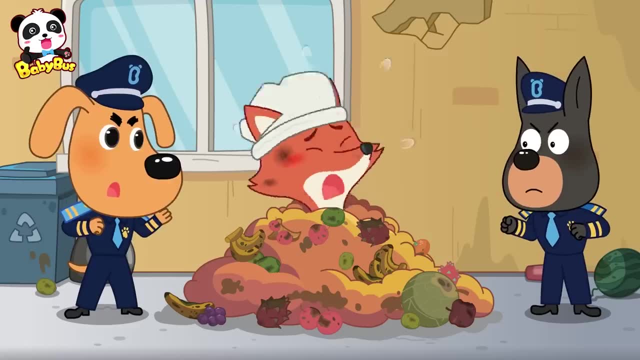 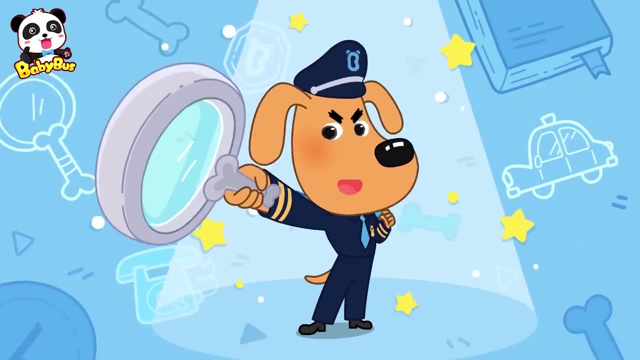 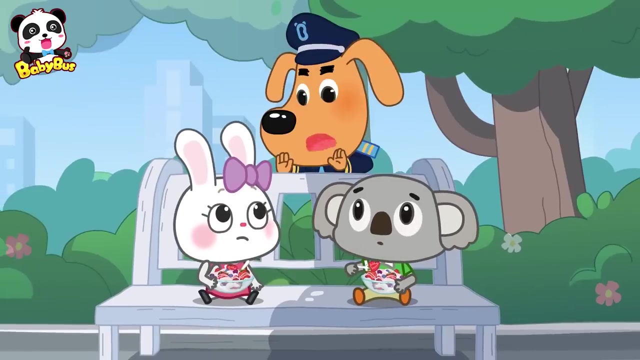 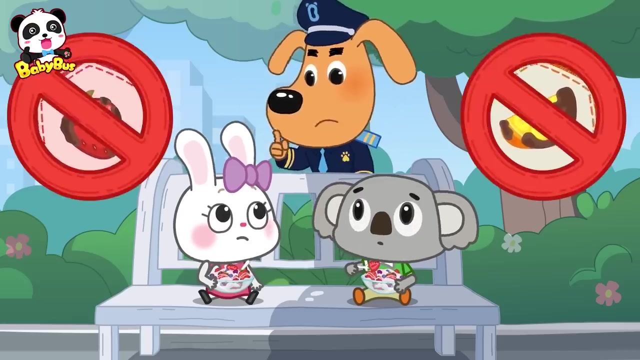 You're going home, Do you? you're so bad you were going to the police station with us. Sheriff Labrador, safety, talk Kids. Check your food before eating. if it looks dirty or rotten or it's past its expiration date, You shouldn't eat it. Rotten food can cause stomachache and even food poisoning. Please keep these in mind. 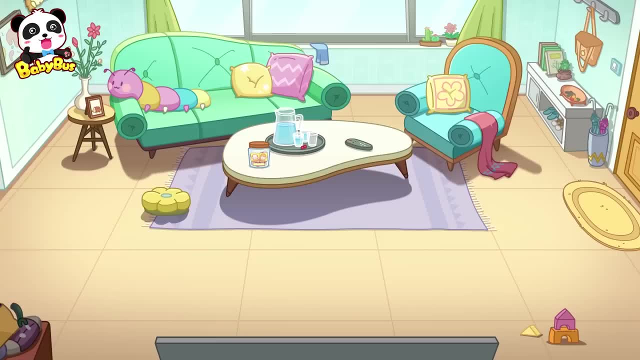 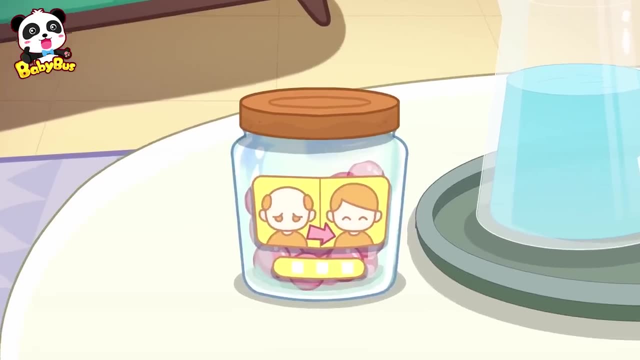 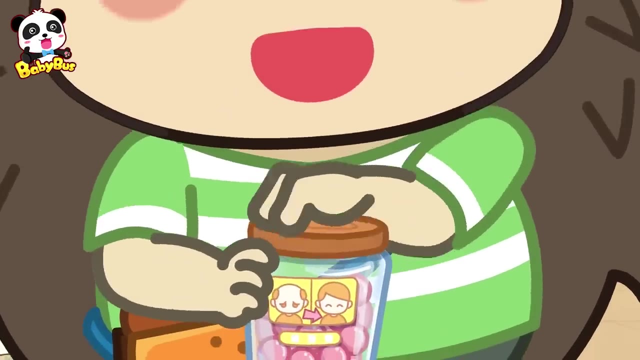 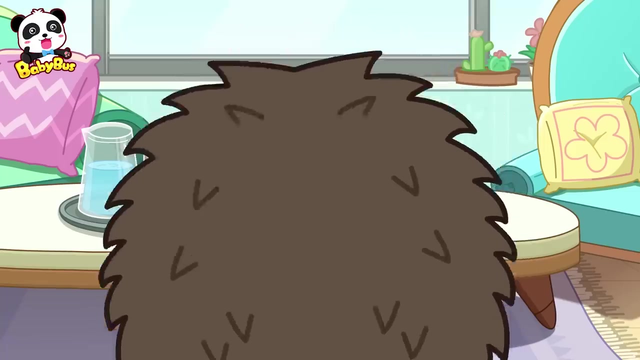 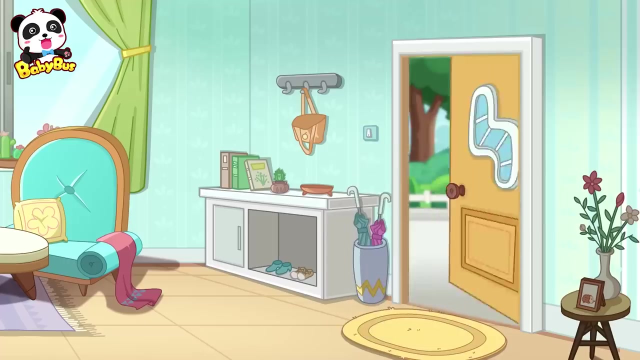 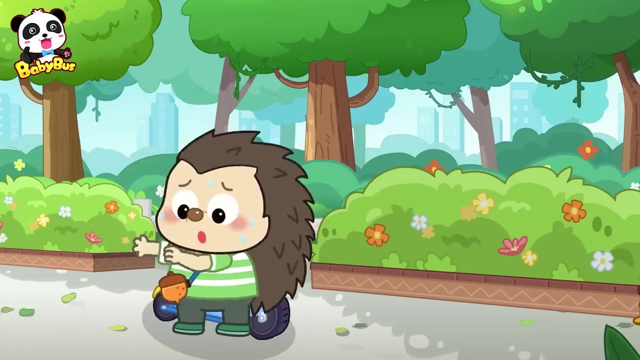 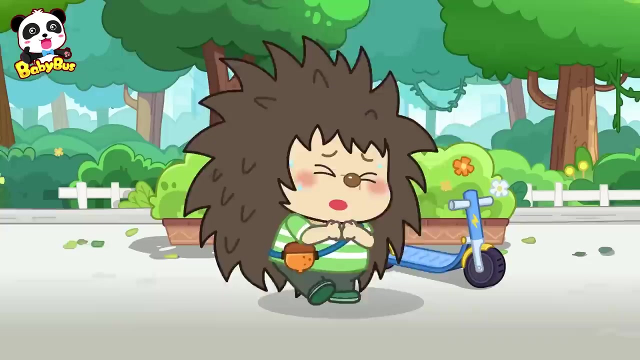 Medicine is not candy. It must be new candies mommy bought. Oh, It tastes strange. Oh well, time to go play. Yoo hoo, Yoo hoo. I'm so itchy. What's happening to me? Huh, My hair. Why is it suddenly growing? 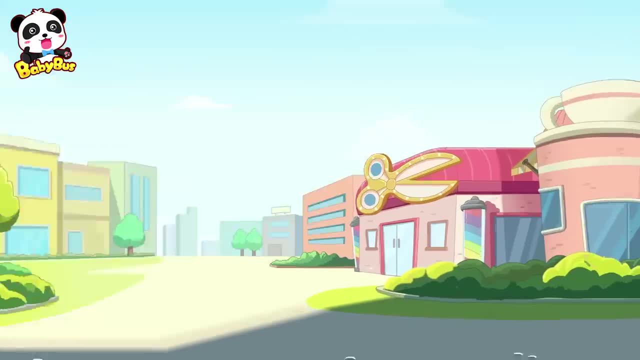 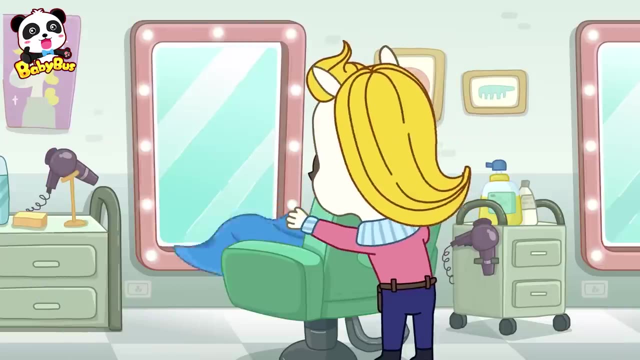 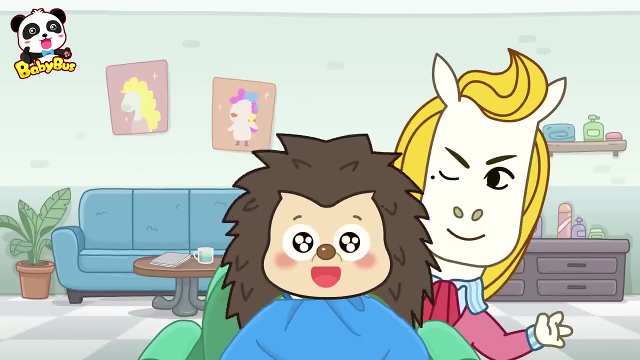 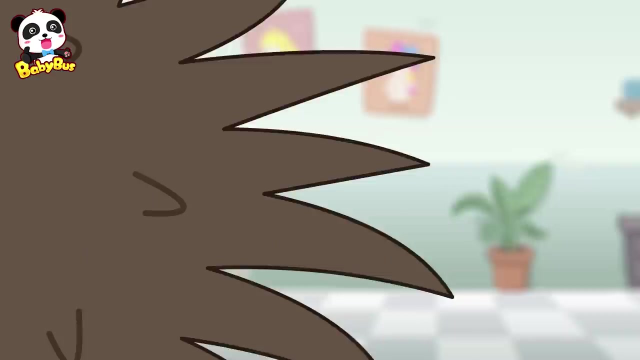 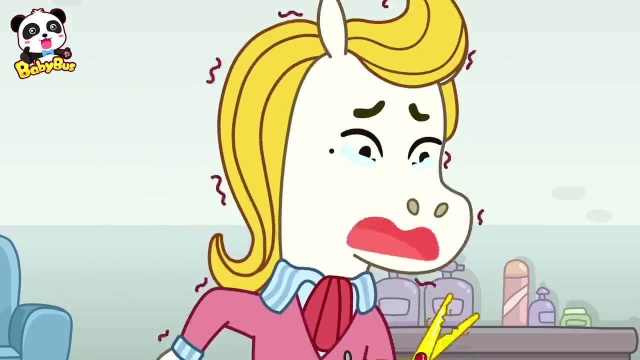 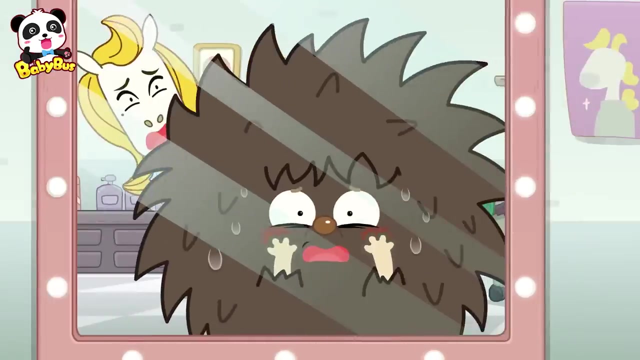 What's going on? Huh, A hair salon. Hmm, leave it to me, I'm gonna make you look stunning. What's going on? I can handle that. My golden scissors- Huh, My hair. What's going on? What happened to me? 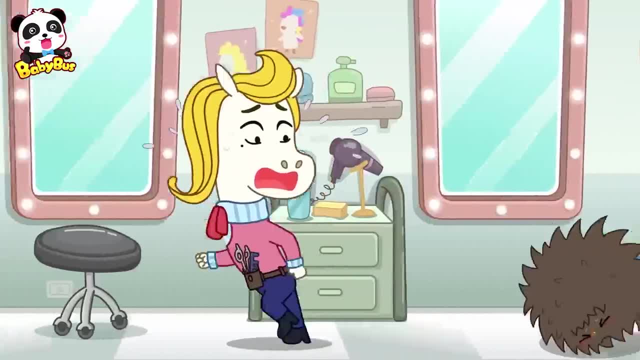 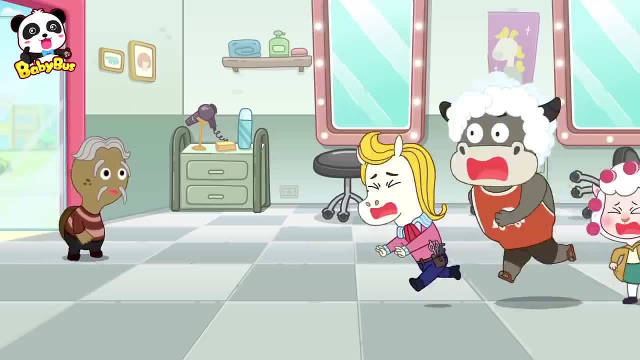 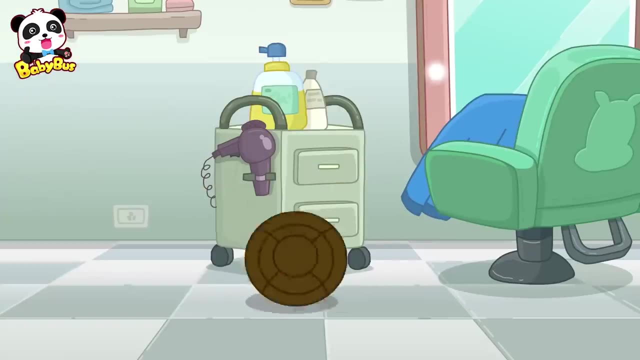 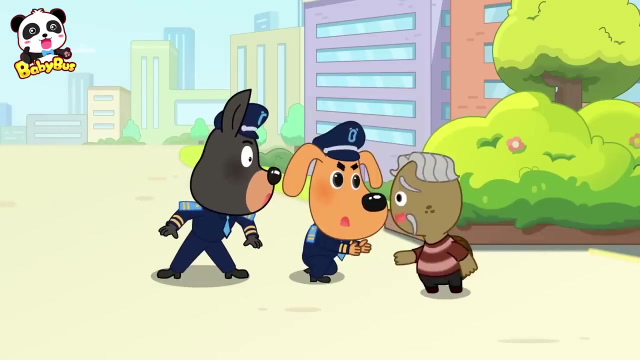 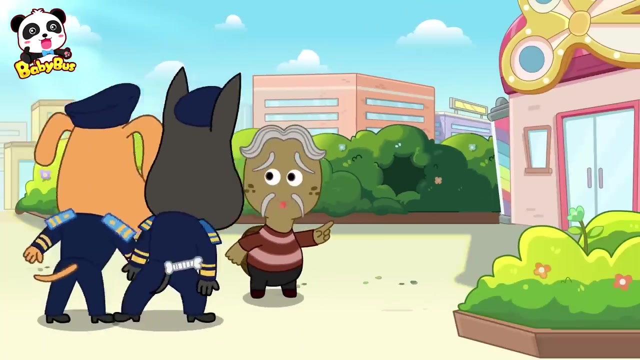 Owww, Boss Run, Uh Huh, Ahhhh, Ah, Oh yeah, Huh, Something's wrong. Sheriff Labrador, a hairy monster was chasing us. A hairy monster, Mm-hmm, It was so scary it went that way. 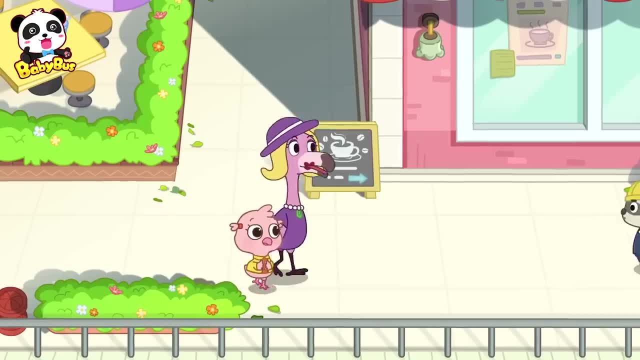 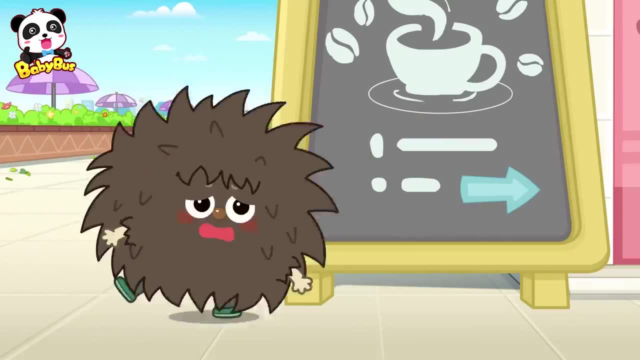 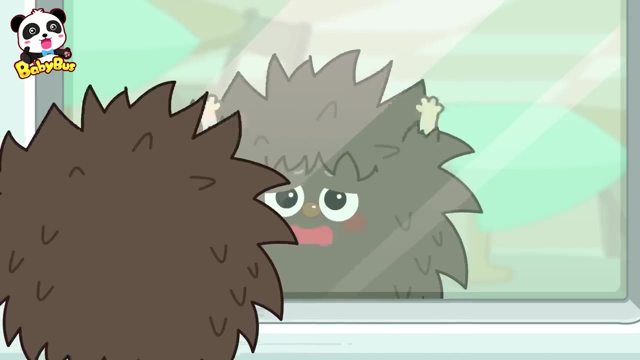 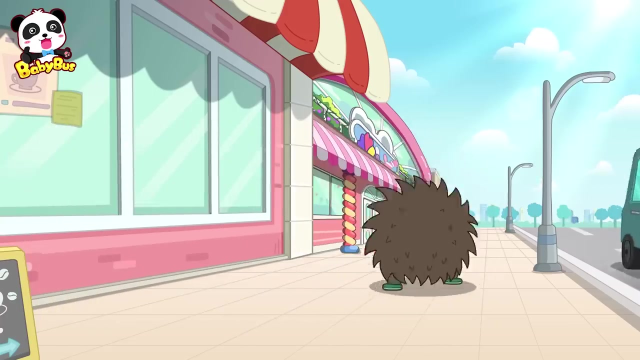 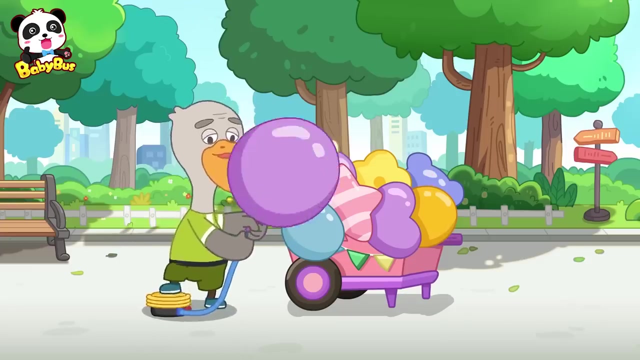 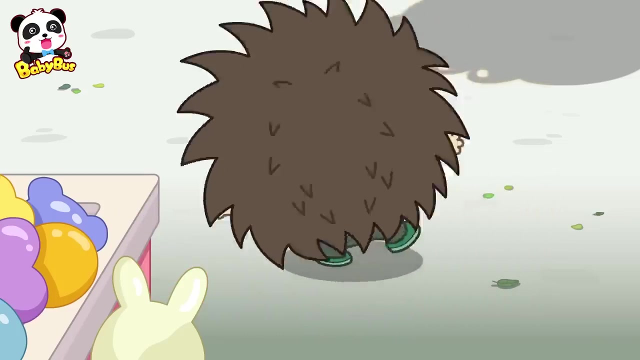 Let's go. Hey, Oh, Oh, Oh, I don't understand What happened to me. My friends won't recognize me. Ha-ha Balloons, Big balloons, Oh, Oh, Oh, I'm sorry, oh. 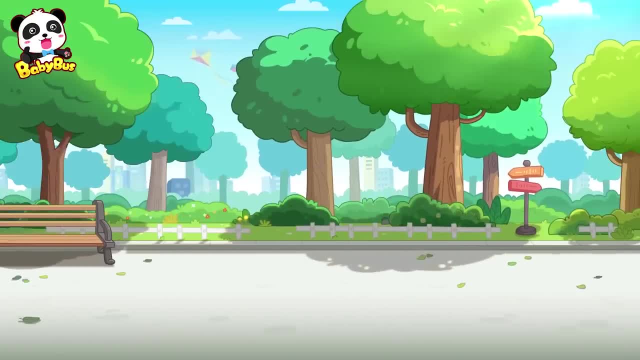 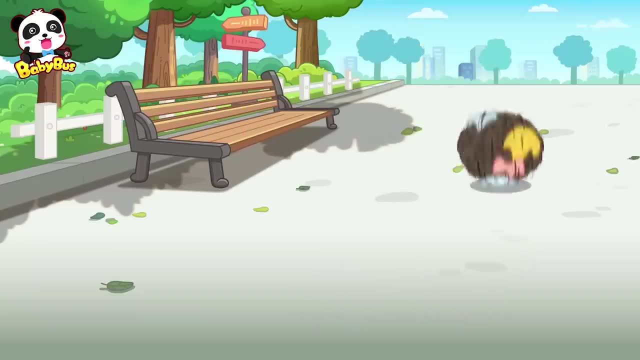 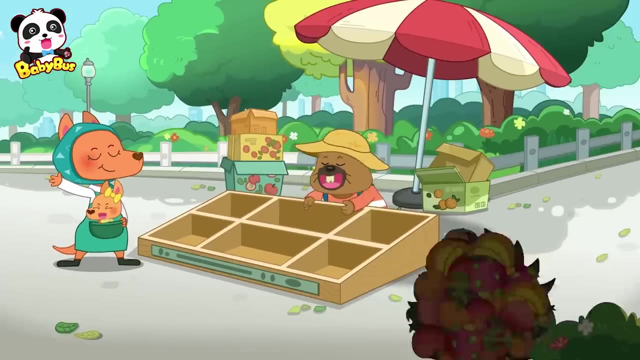 Stay away. I didn't mean it. Oh, Oh, Oh, Oh, Oh, Oh, Mommy, I want this, this and this too. Please wrap everything up for me, All right, That way, Oh Oh. 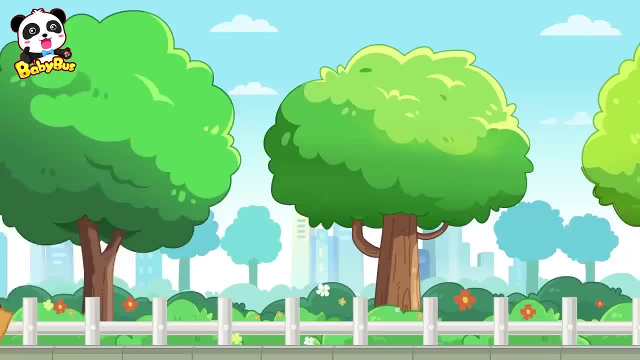 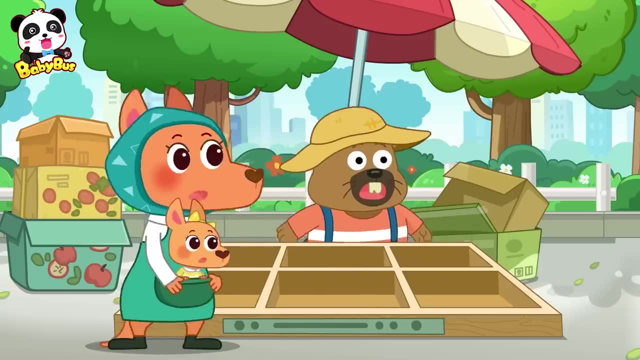 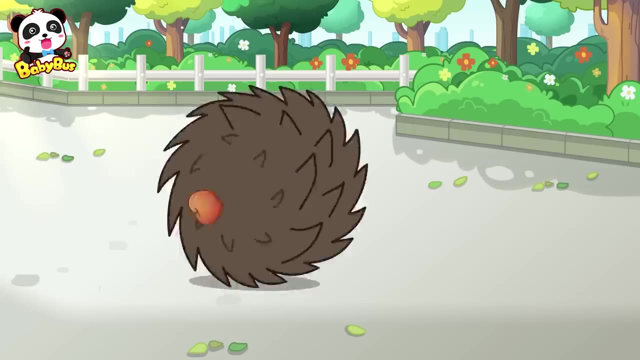 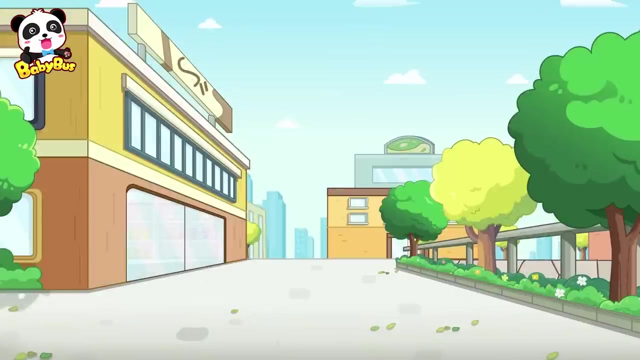 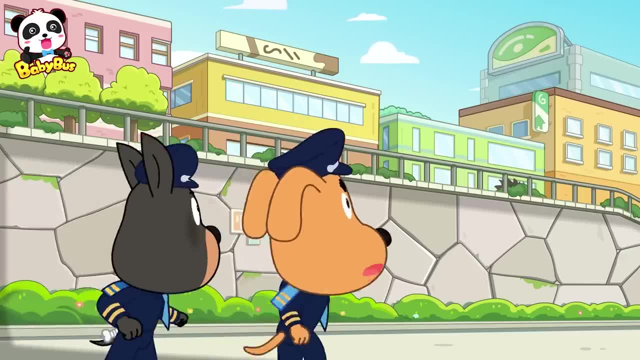 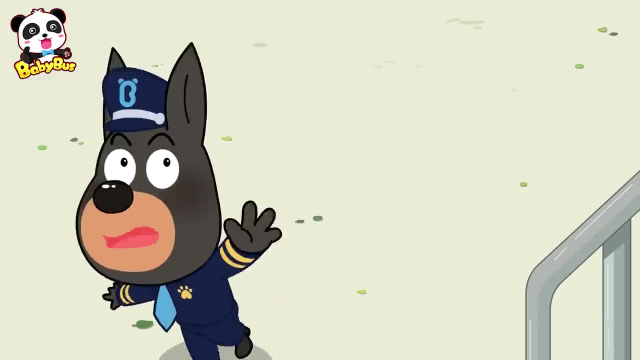 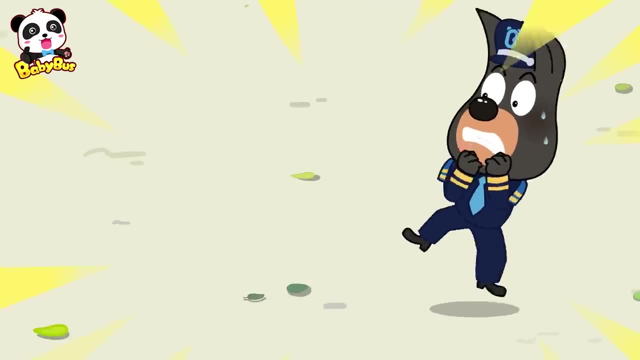 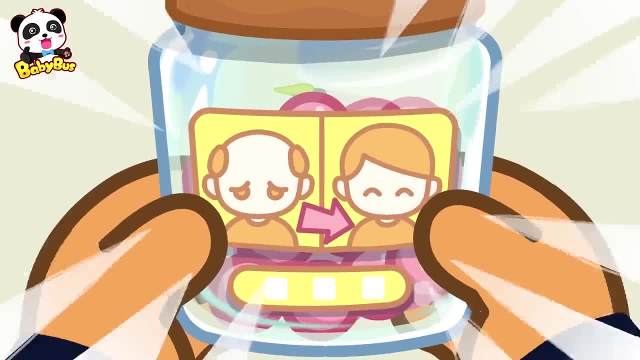 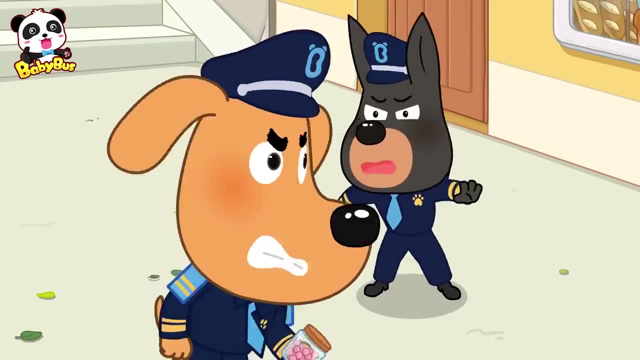 Uh, Uh. What's this? Hair growth pills I got. it. Looks like he took the hair growth pills by mistake. Uh, That's not safe. We need to take him to the hospital. Uh, Uh, Uh Uh. 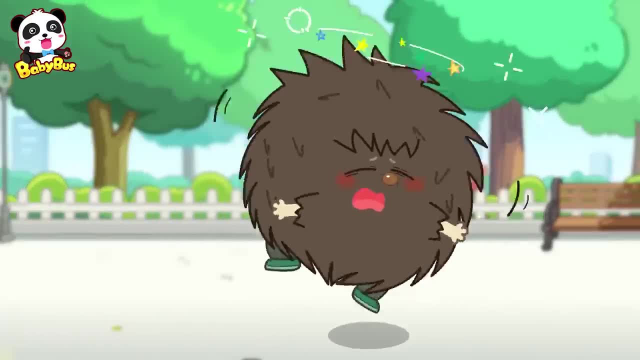 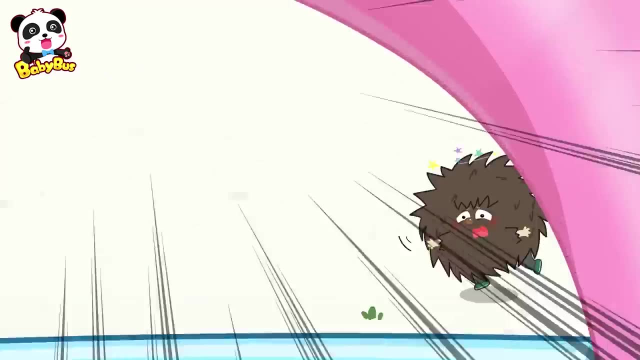 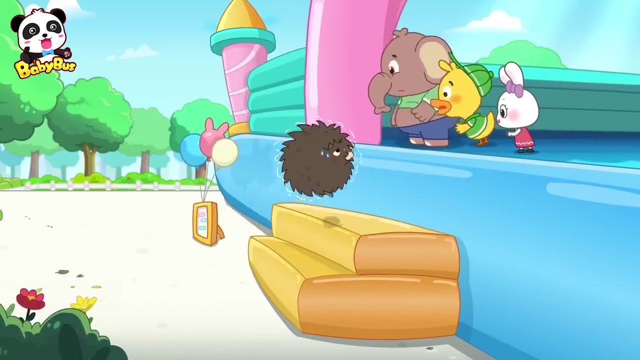 Uh, Uh, I'm so dizzy, Yeah, Ha-ha-ha. Oh, Why is Little Hedgehog not here yet? Uh, I'm here. Oh, Uh, Little Hedgehog, What happened? Uh, Uh, Uh. 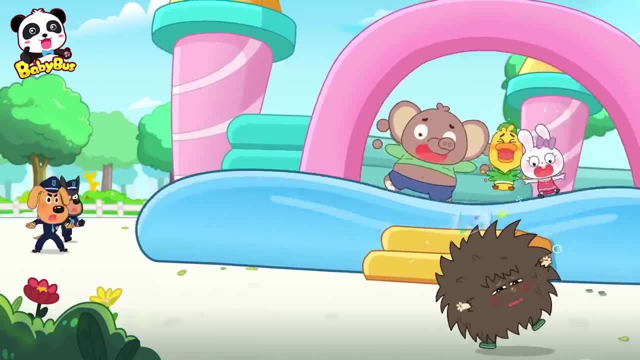 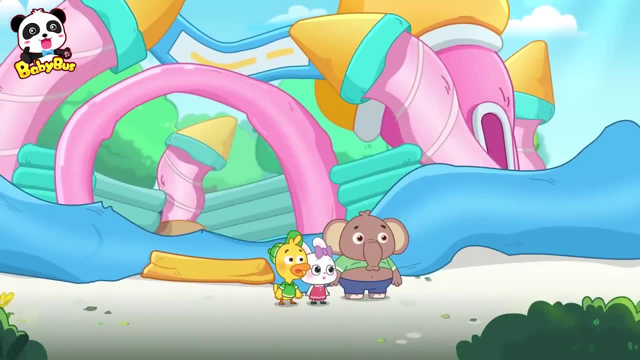 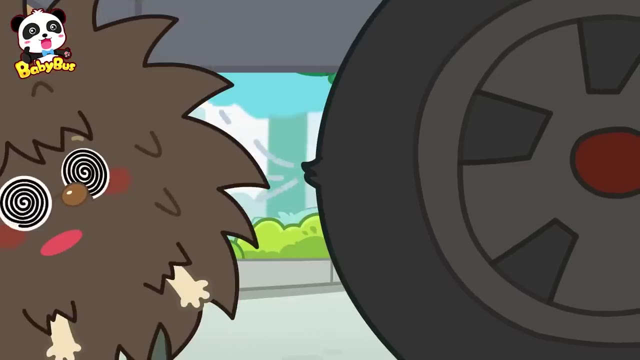 Uh Uh, Uh Uh. Watch out, Uh, Uh, Uh Uh, He's over there. Uh, Uh-oh, Uh-oh, Uh-oh, Uh-oh, Uh, Uh-oh, Uh Uh. 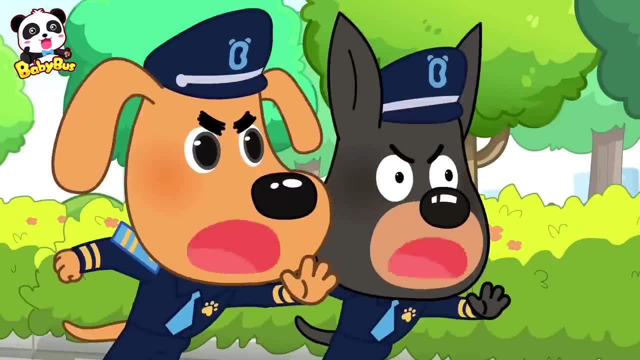 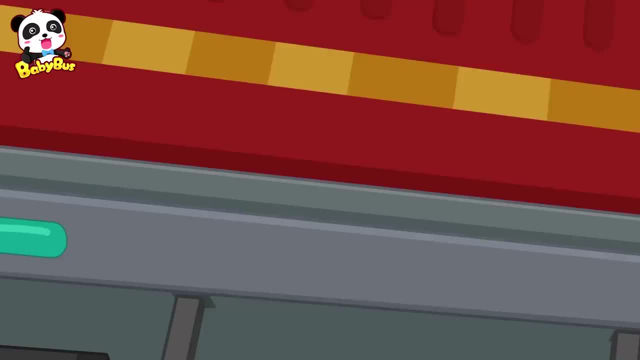 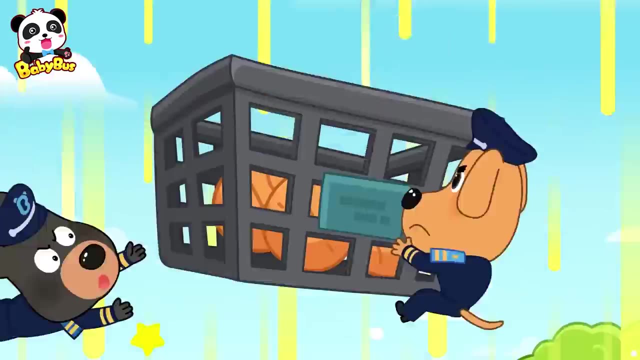 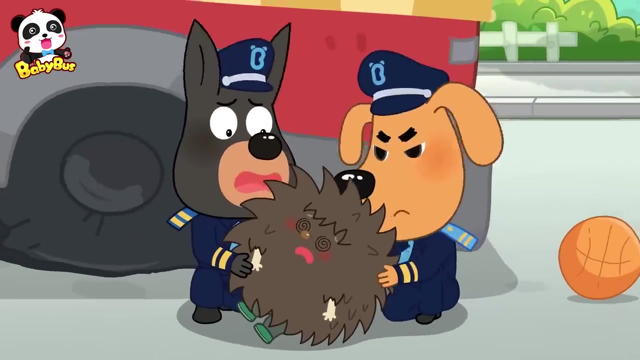 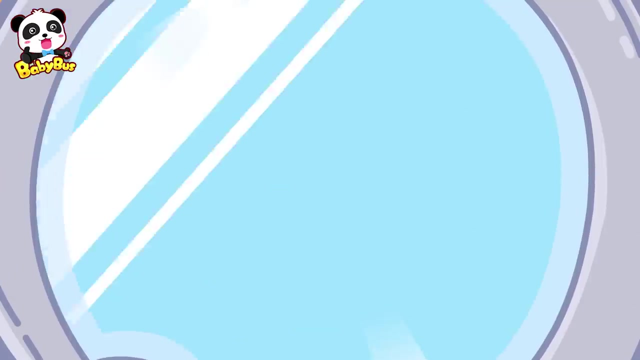 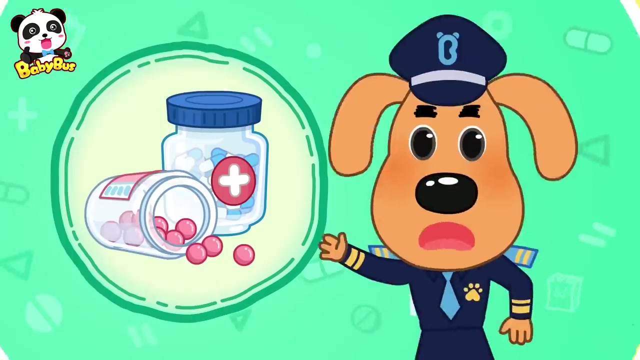 Uh, Ow, Uh-huh, Ah. Watch out, Huh, Huh, Ah, Uh, Uh. Oh. no, My bottom Little Hedgehog. Take him to the hospital. Sheriff Labrador's Safety Talk. Kids, be careful not to eat medicine like it's candy. 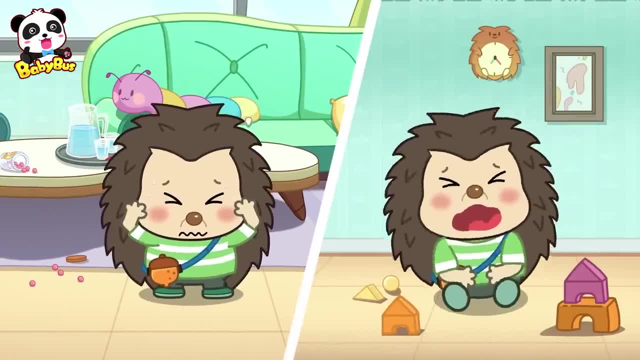 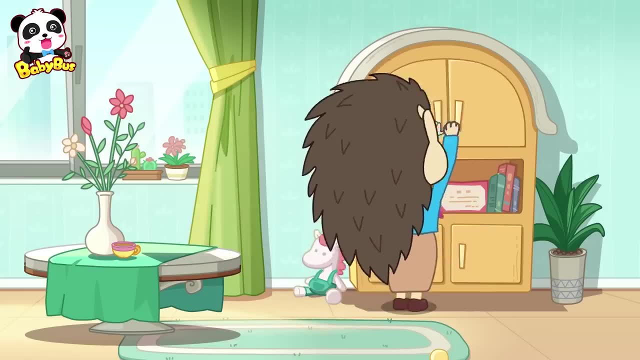 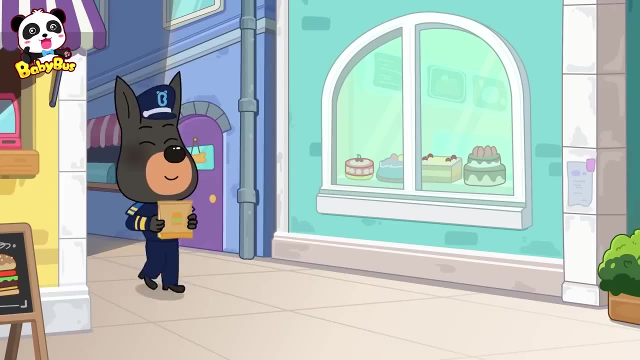 You might feel dizzy, get a headache or even a stomach ache, and your life might even be in danger. Also, parents should keep medicine out of the reach of children. Please remember that Woof Fake Child, Mmm Ha-ha, It looks so yummy. 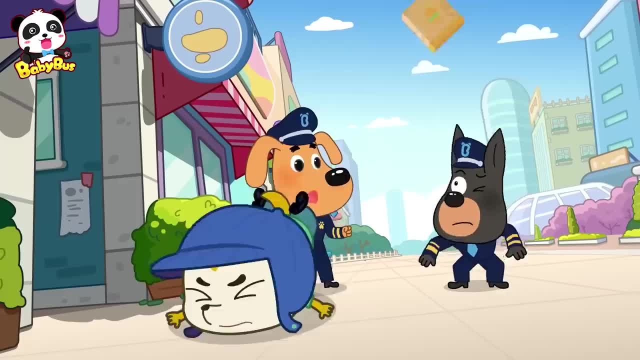 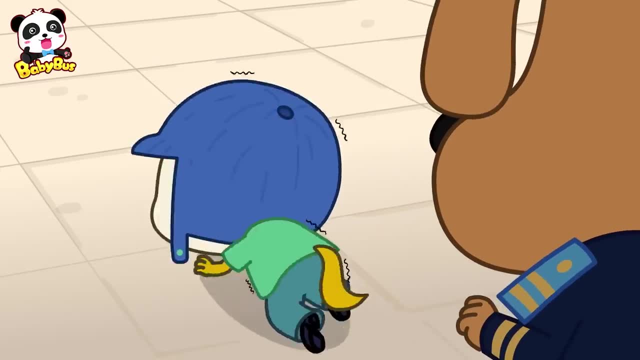 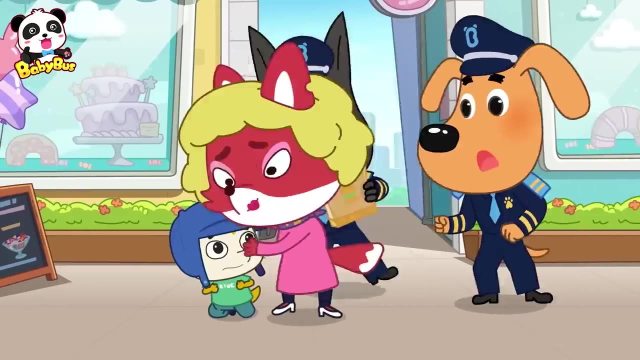 Mmm, Ah Ow. Hey, kid, are you okay? Watch where you're going. Oh, Police, They don't know, They don't know. Oh, Oh, no, Little Fox, My child Mari's been looking for you. 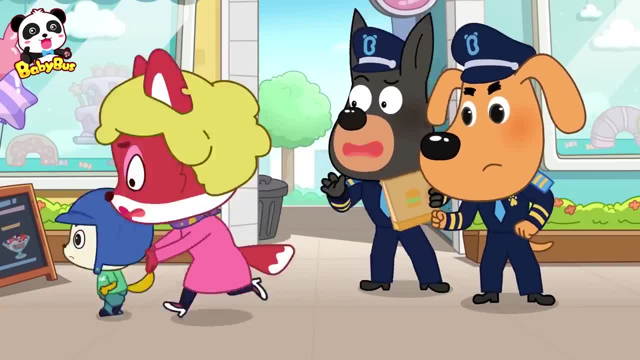 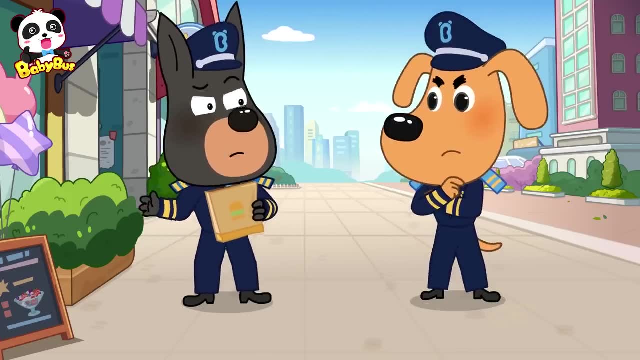 Why are you here by yourself? Thank you, police officer. Bye, They're acting weird, Isn't it strange? There might be something going on. Let's follow them. Watch out, Gah, All right. Oh my God. 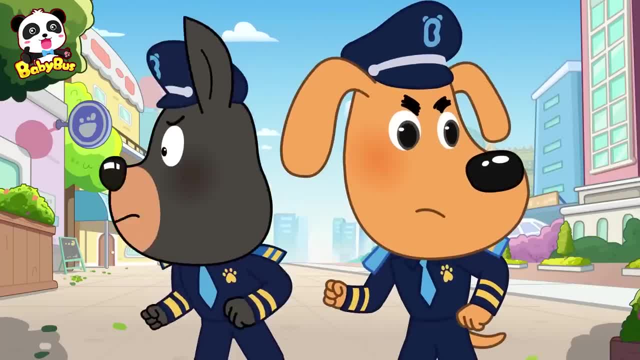 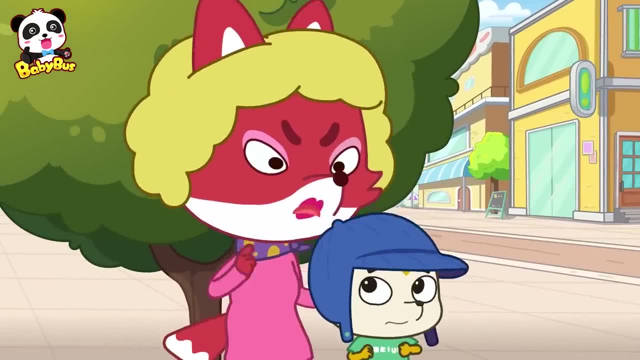 They're going the same way. They're gone. Oh no, Where did they go? Let's go that way. Hey, Hey, Huh, Hey, Hey. we almost got caught by the police. Stop nagging. We need to find a child to kidnap today. 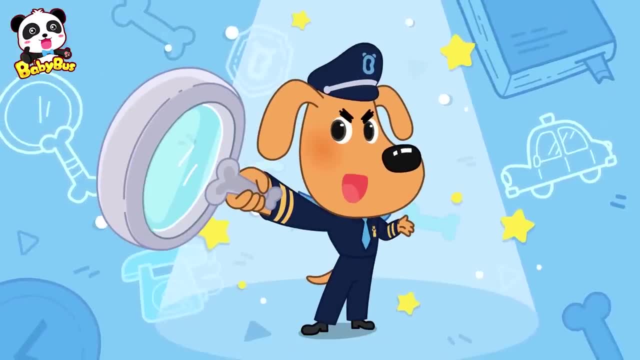 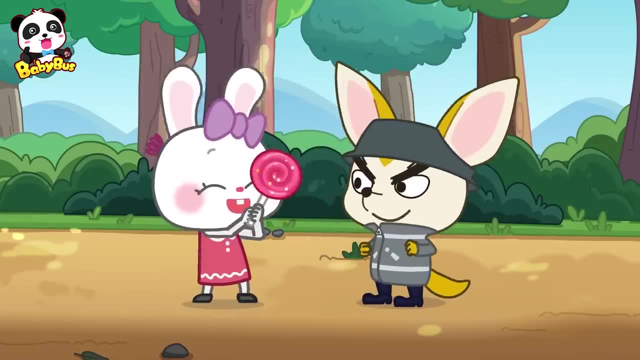 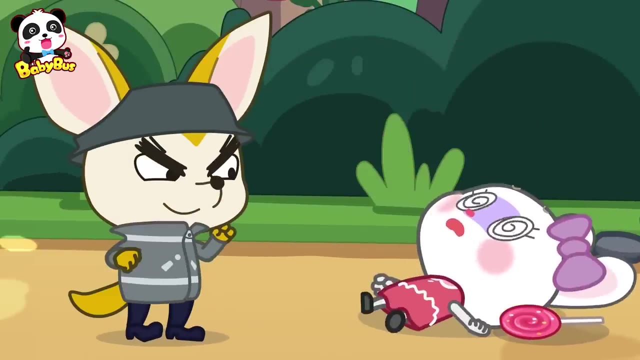 Sheriff Labrador's Safety Talk: Kids: you should beware of strangers. Even if it's a kid, you should always be careful of who you meet. Never take anything they give you and never go with them, Because they could be with other kidnappers. 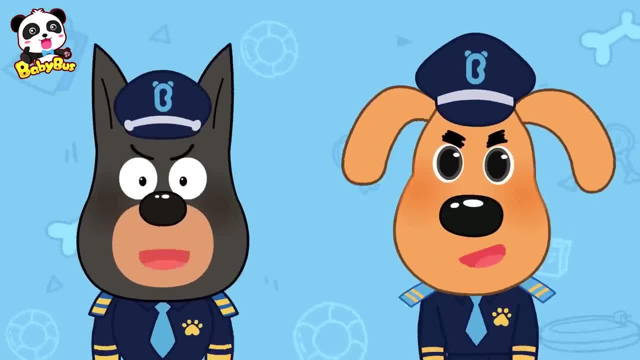 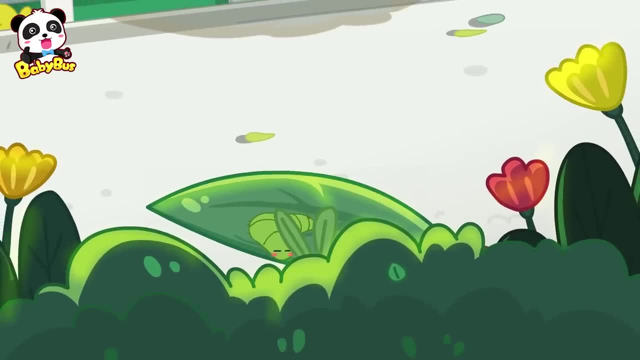 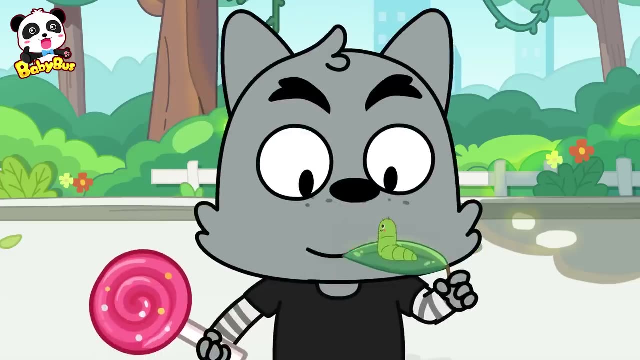 Please remember that Never play with caterpillars. Do-do-do-do-do-do-do-do- Huh, A caterpillar, It looks funny, Huh-huh-huh-huh-huh-do-do-do-do-do-do Ouch. 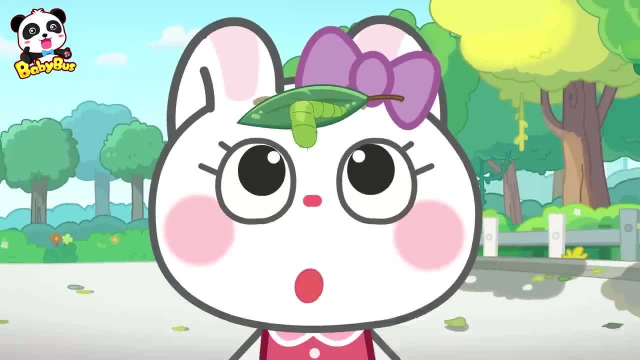 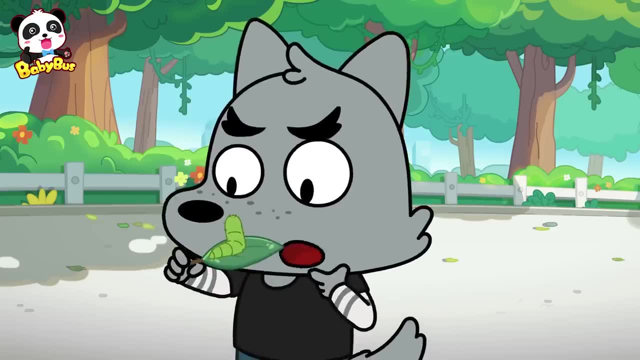 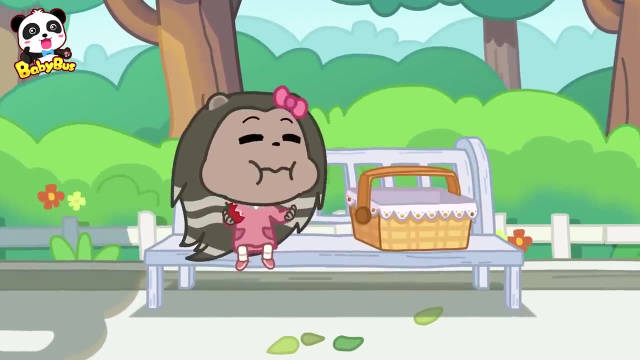 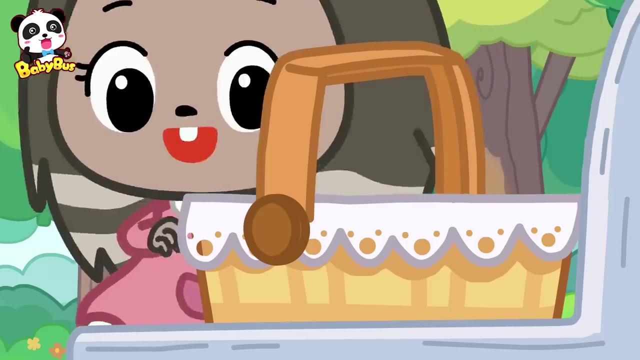 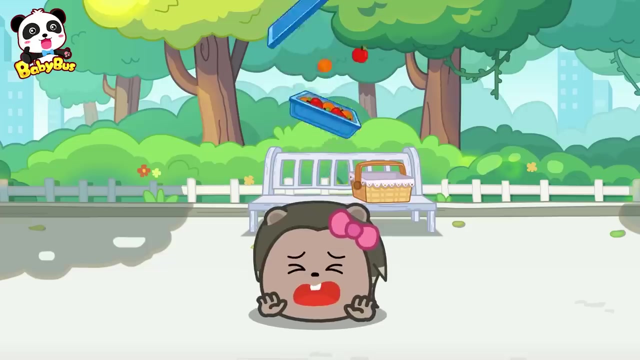 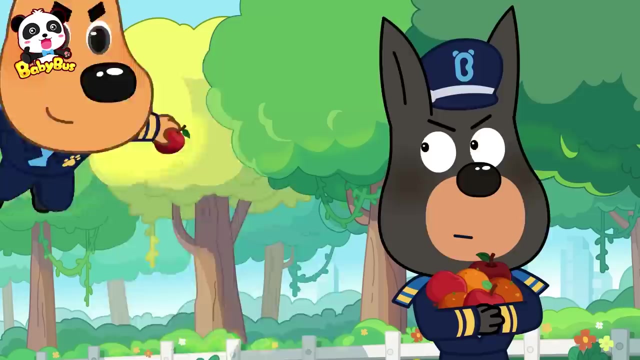 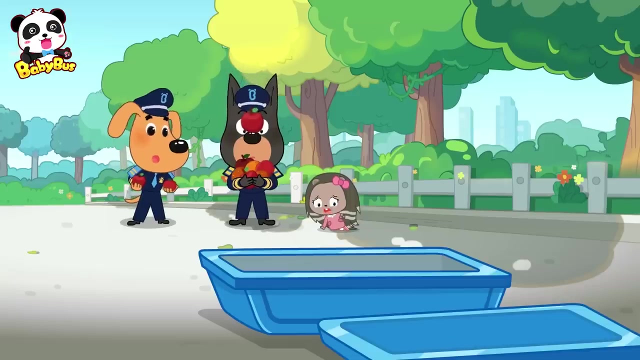 Uh, Huh, Huh, Huh, A caterpillar. Huh, Aren't they all scared of caterpillars? Ouch, Ouch, Sheriff Labrador, so many caterpillars are in there. It's really scary. 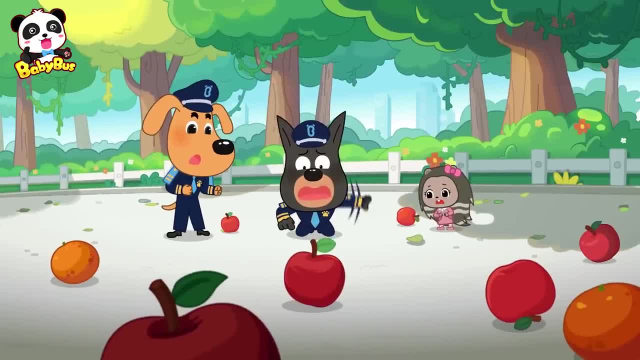 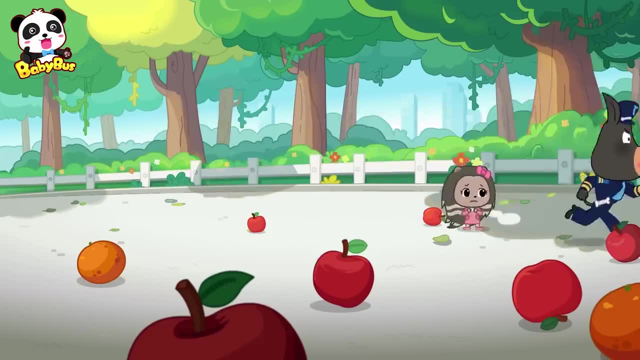 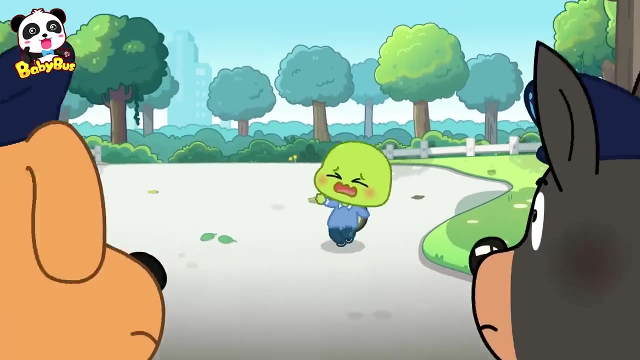 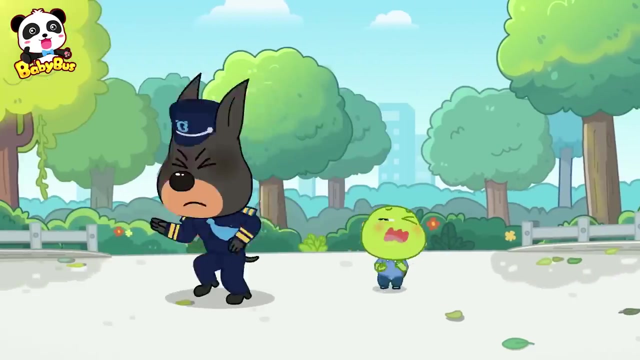 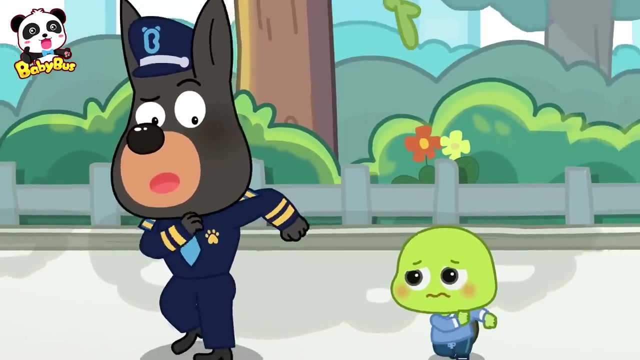 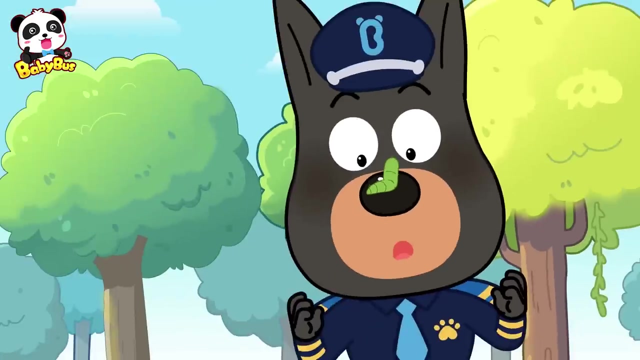 A caterpillar. Let's go Over there. Hey Little Little, Little turtle, Are you okay? I'm so itchy It feels like something's under my shell. So itchy, So itchy- Another caterpillar. 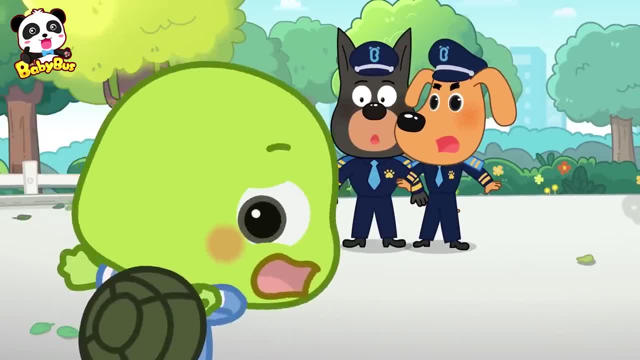 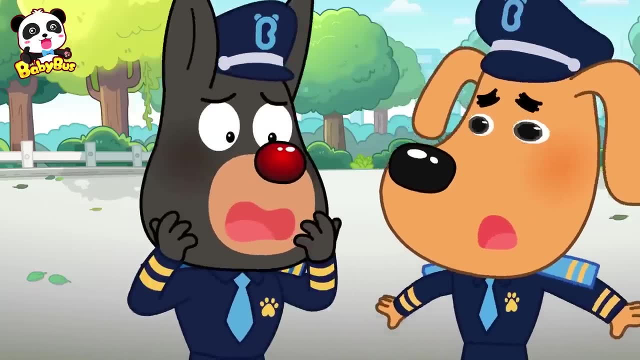 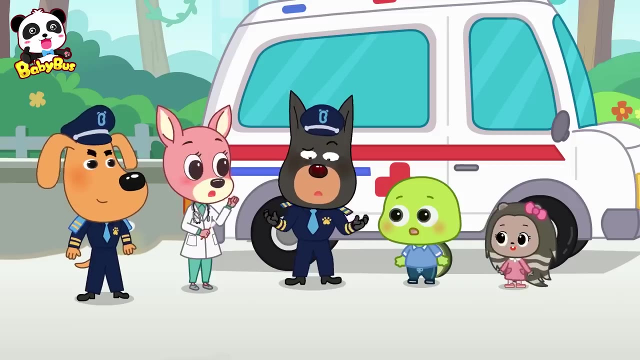 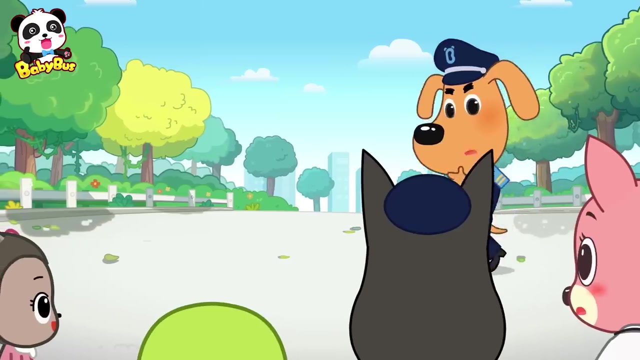 Oh, my neck, My nose, Oh no, The caterpillars are venomous. The treatment is all done. You'll feel better soon. Caterpillars usually live in the woods. They won't leave there by themselves, unless someone moves them on purpose. 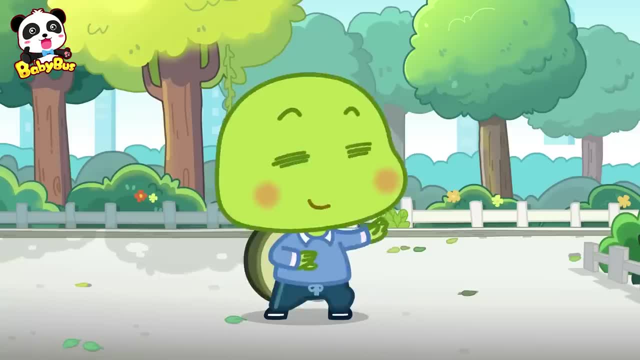 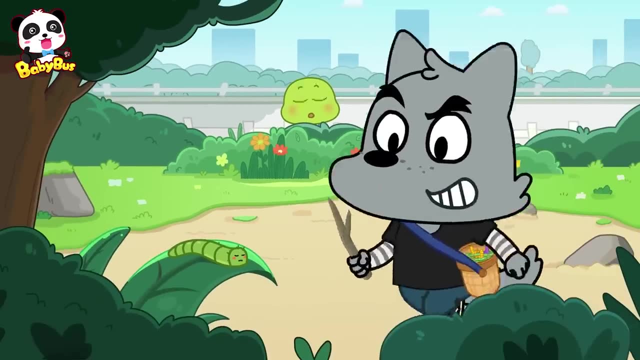 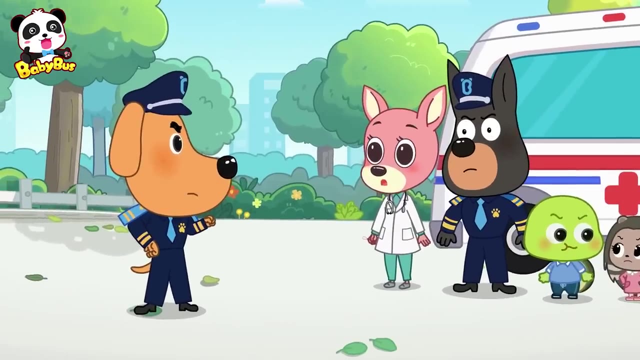 Oh, I remember When I was doing Tai Chi this morning I saw a little wolf catching caterpillars in the bush Little wolf must be scaring people with caterpillars. We need to stop him now. Oh, Oh, Oh. 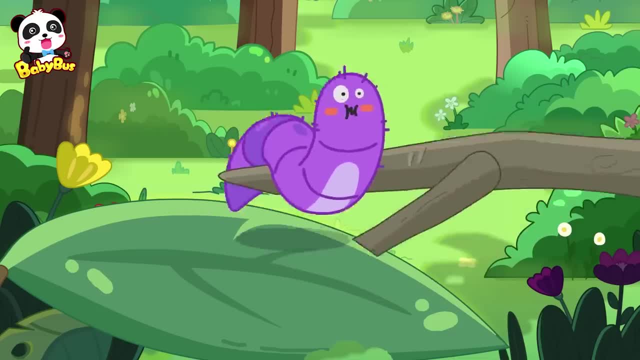 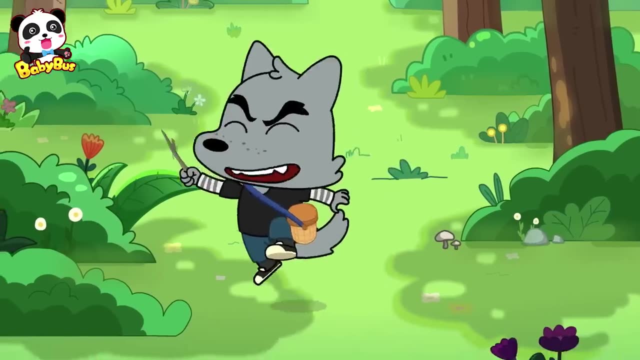 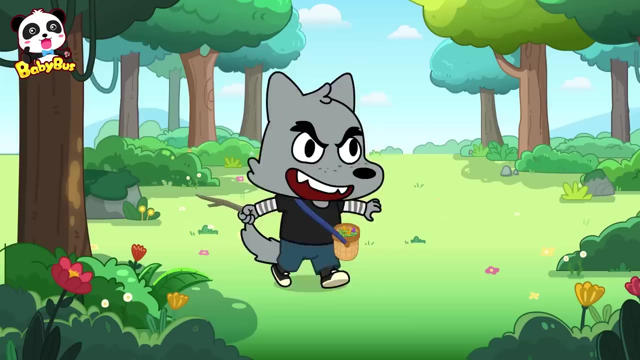 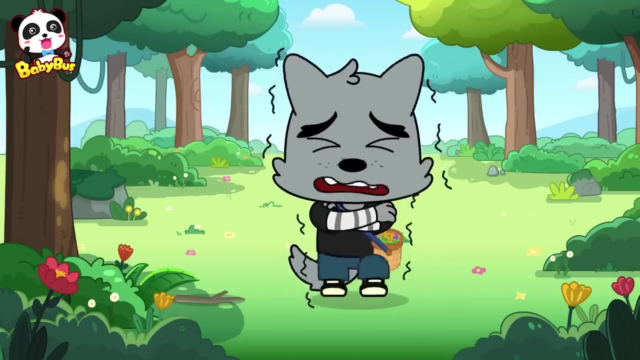 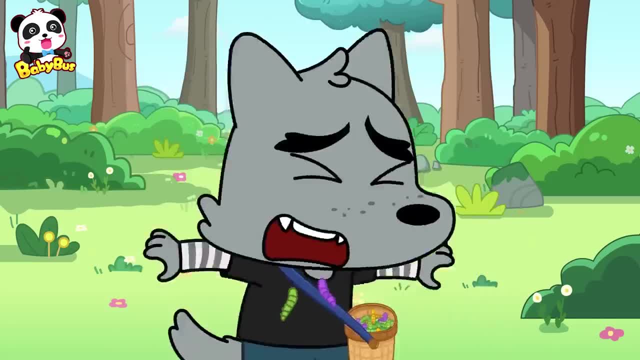 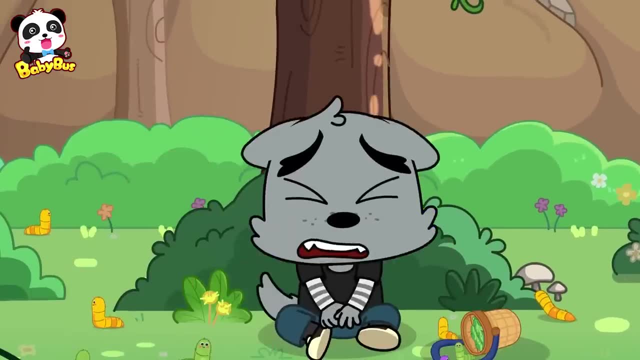 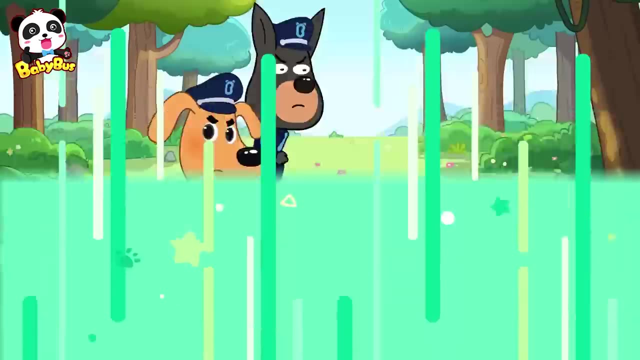 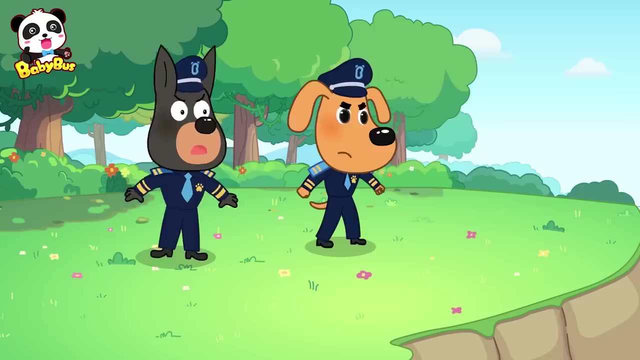 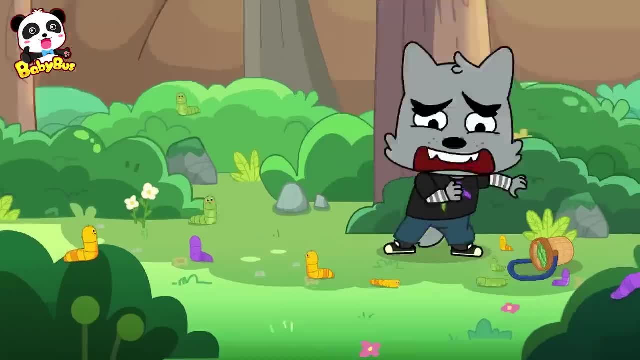 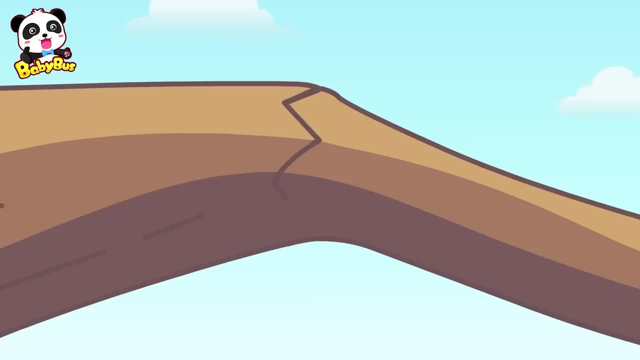 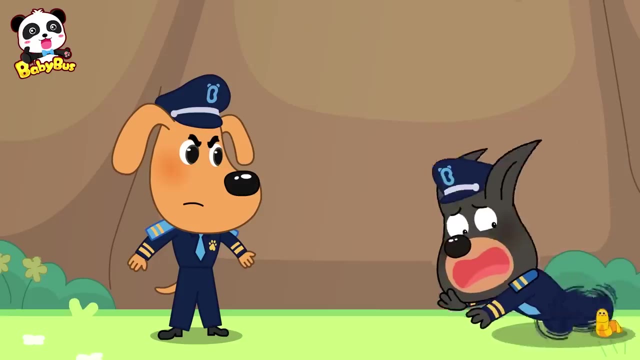 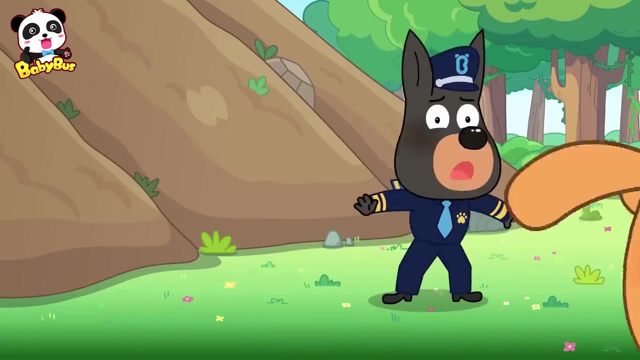 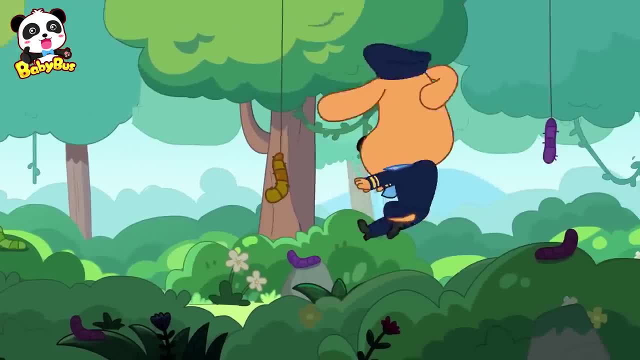 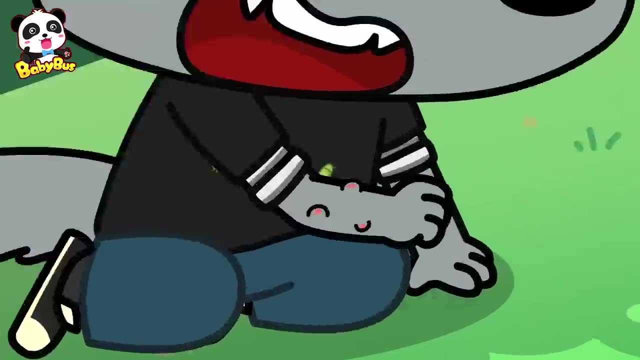 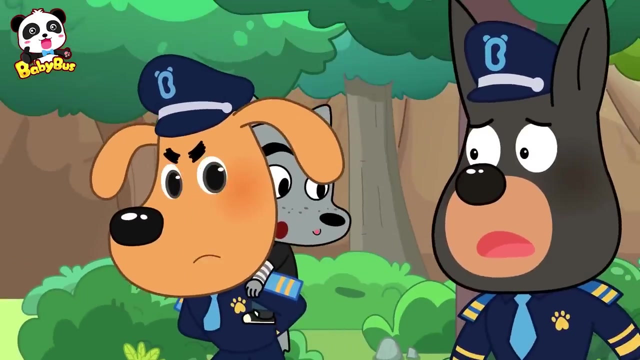 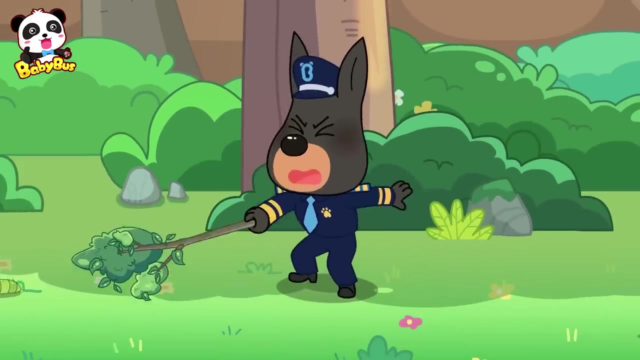 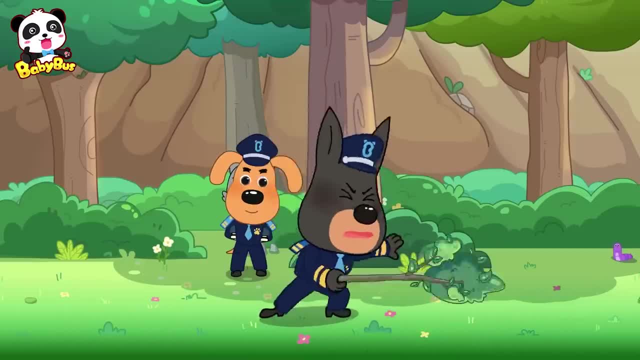 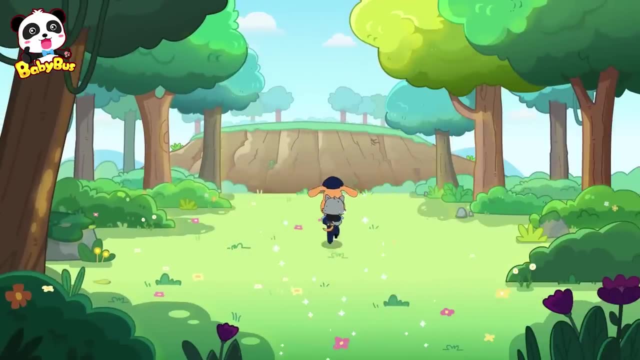 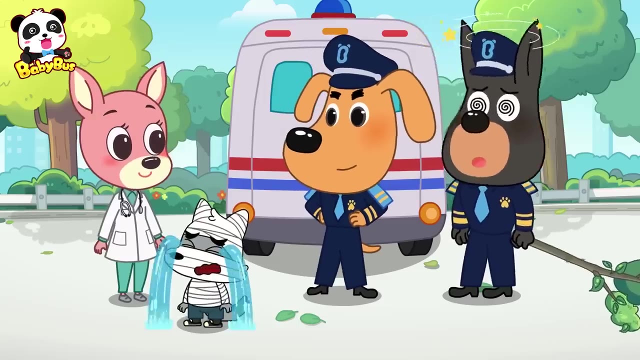 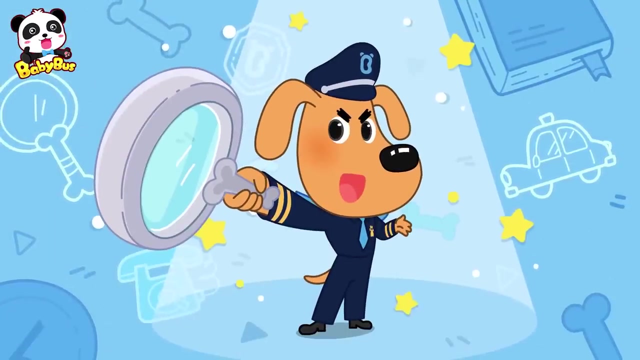 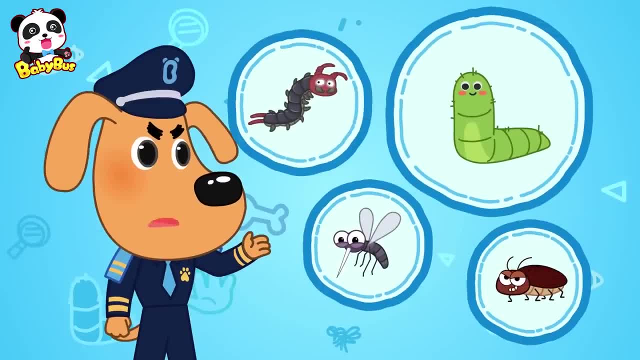 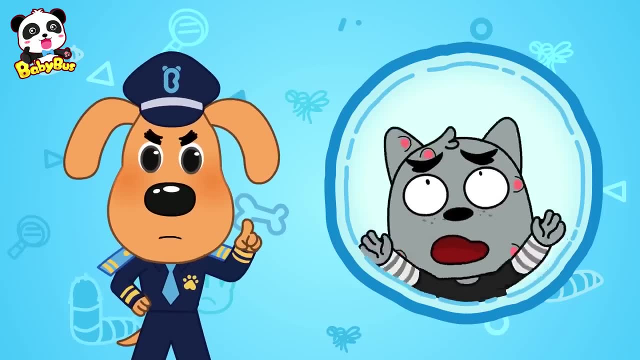 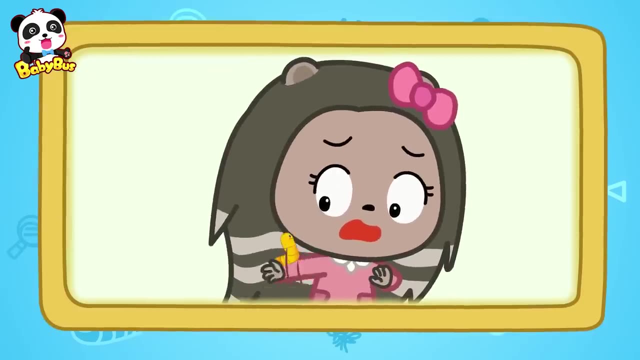 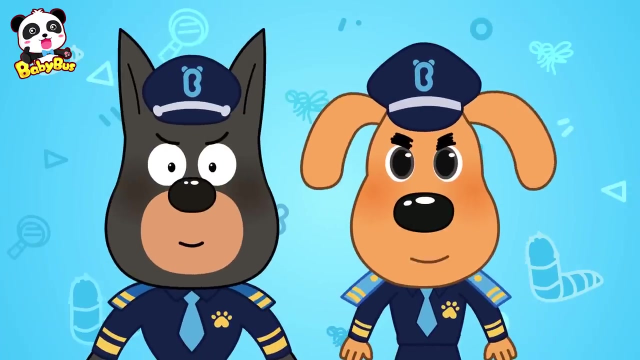 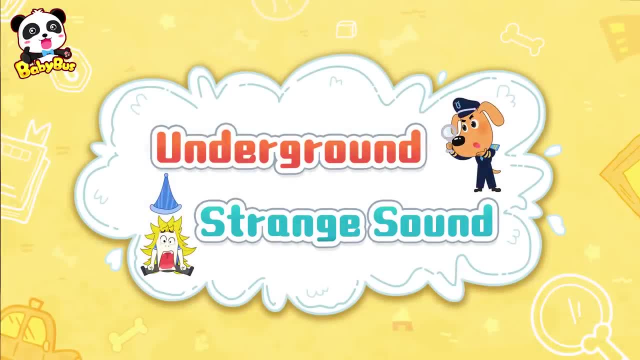 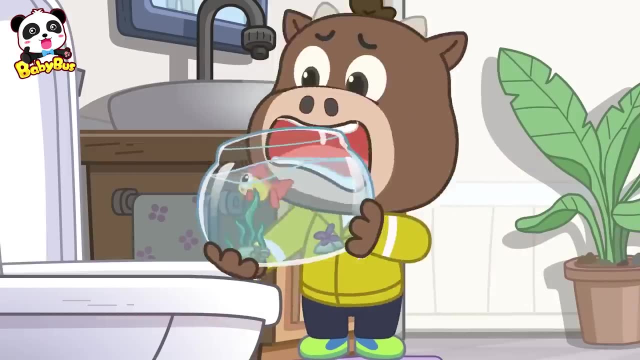 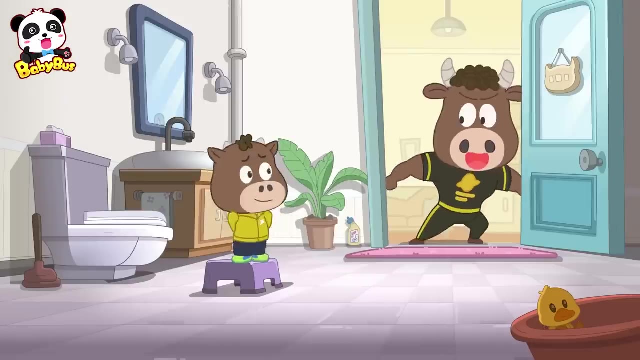 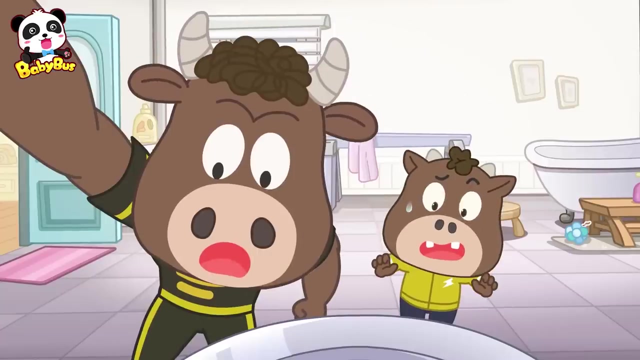 Woof, Underground strange sound. It's a big monster. Sweetie, It's Daddy. Are you there, sweetie, Playing around with the toilet again? No, I'm not, Let's go. It's time for bed, Let's go. 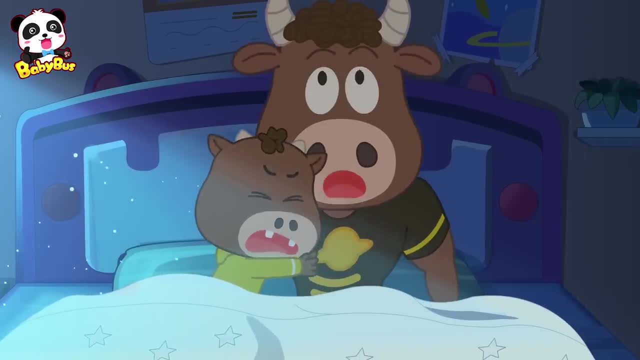 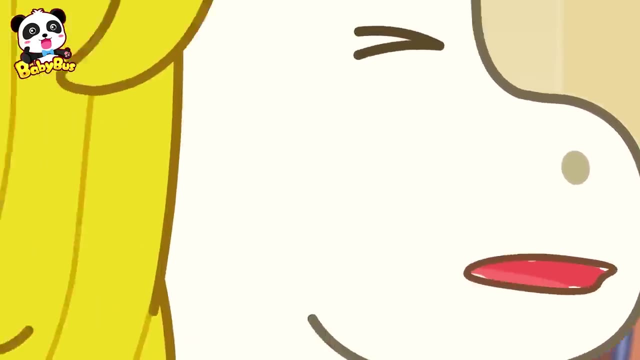 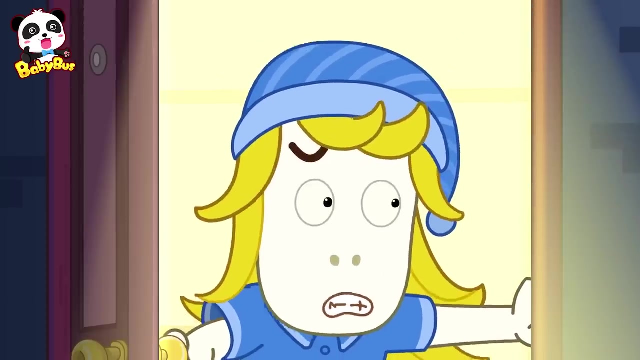 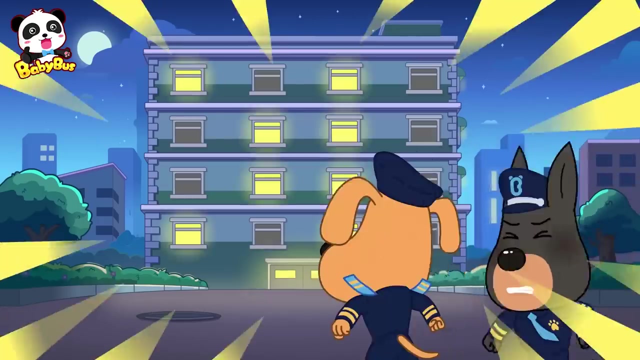 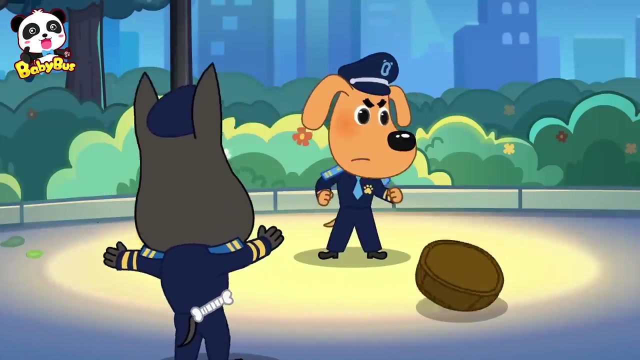 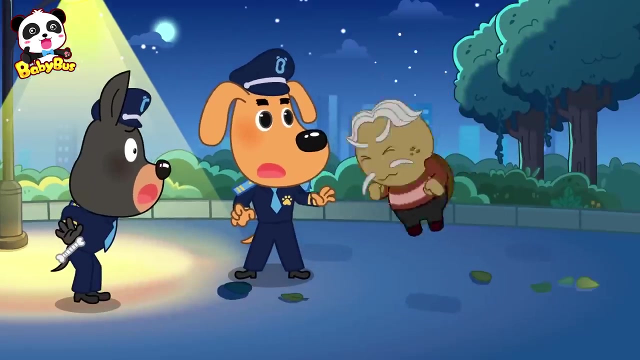 Daddy, Daddy, What's that sound? Who is it? Who is it at this time of the night? It's a ghost. What's going on? There's a ghost in the building. There's no ghost in the world- Dummy. 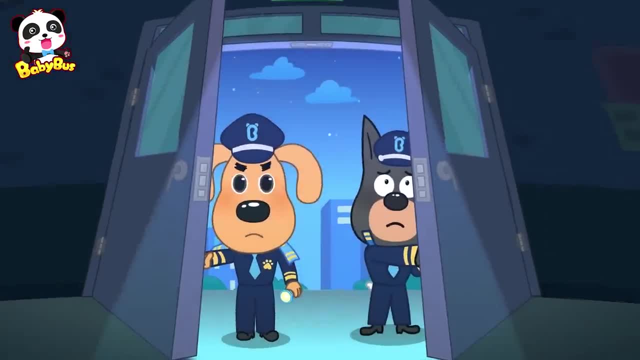 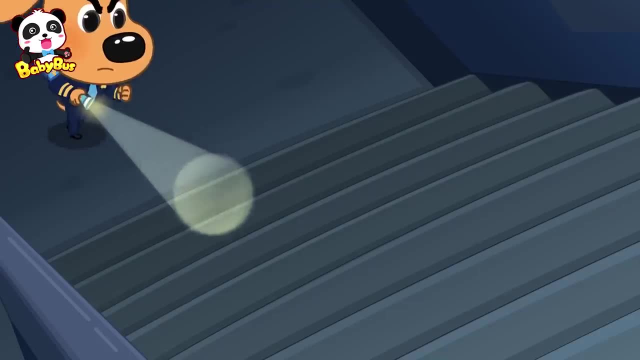 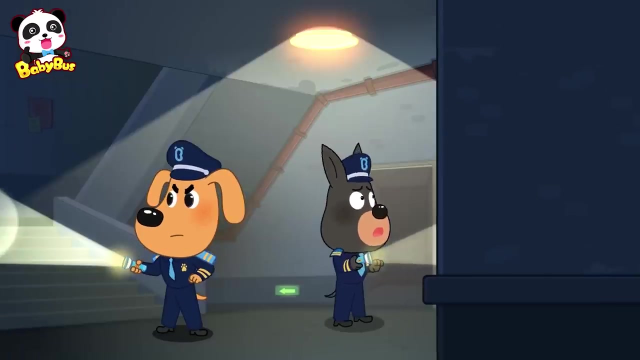 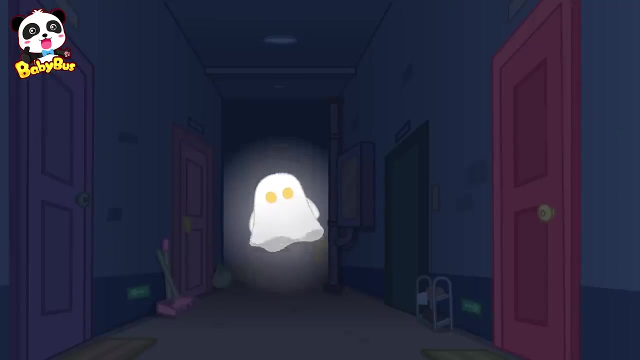 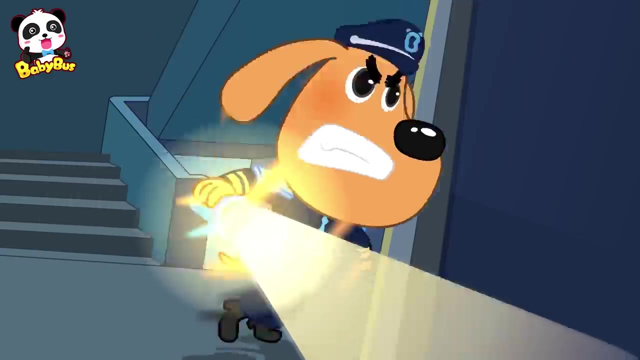 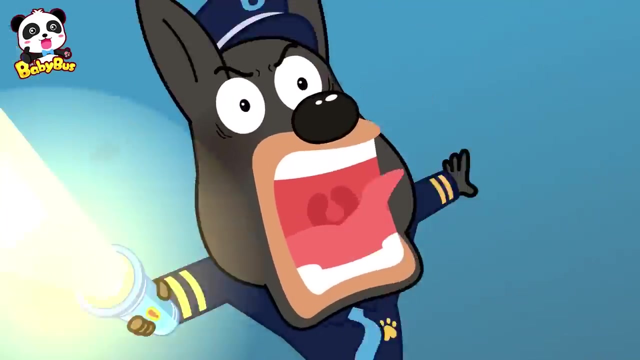 Let's go have a look. Huh, Hmm, Hmm, Huh, Huh, Huh, Huh. Oh, my wishlist. The ghost Hey, Part 2. Who's pretending to be a ghost? Make way, The bear opens the door. 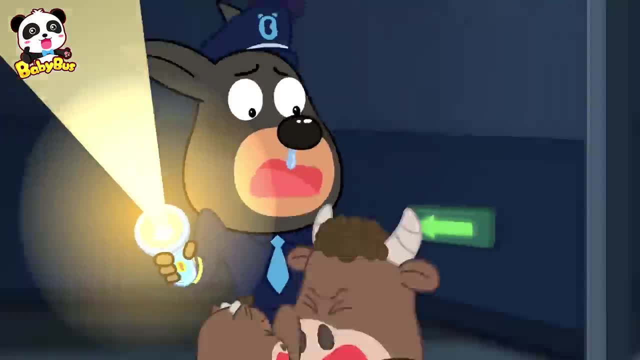 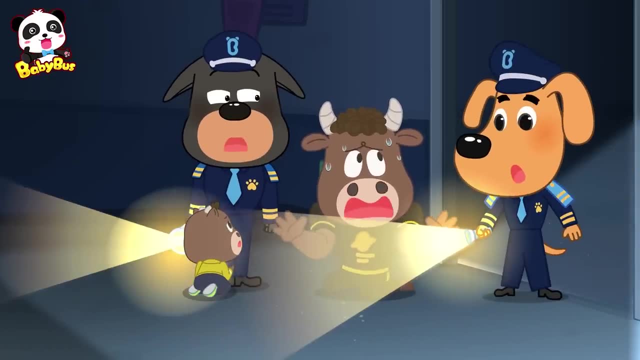 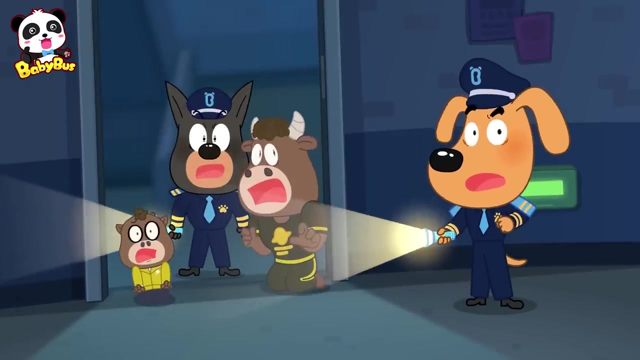 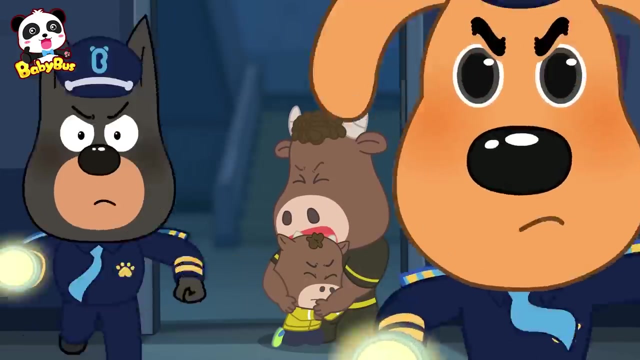 The aquarium opens. eles. This can't end right now. Sorry, we didn't mean to. We heard a strange sound. It was so extraordinary. That's a sound, Joby, let's go. Here's the buffalo's house. 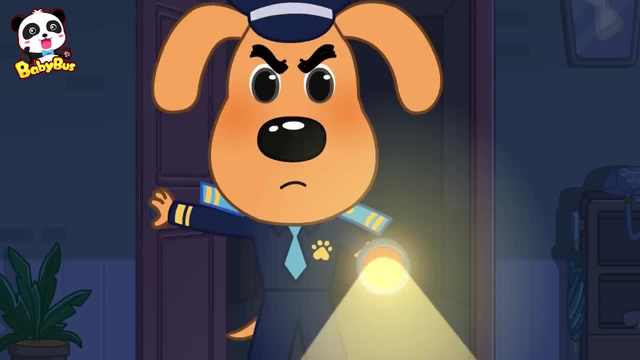 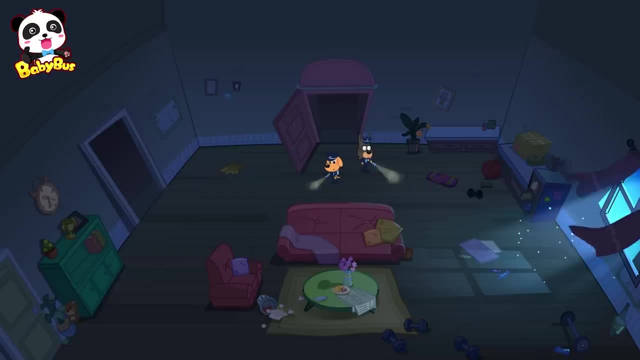 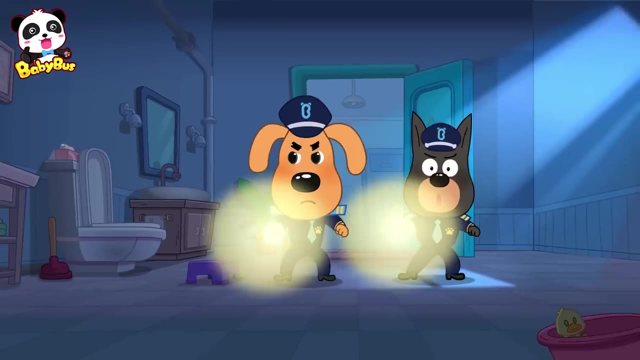 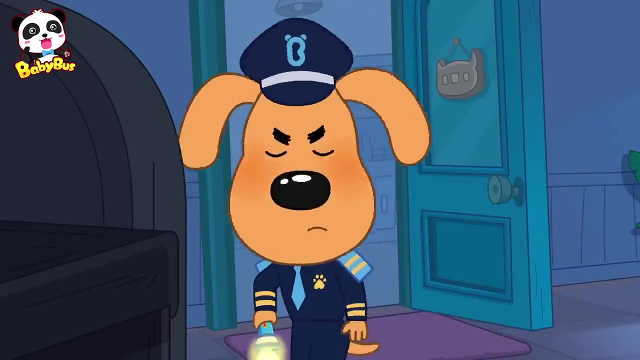 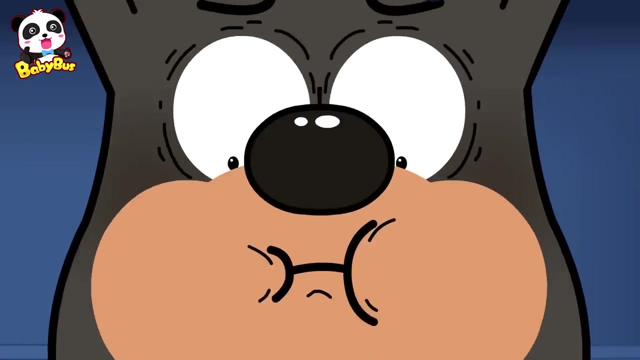 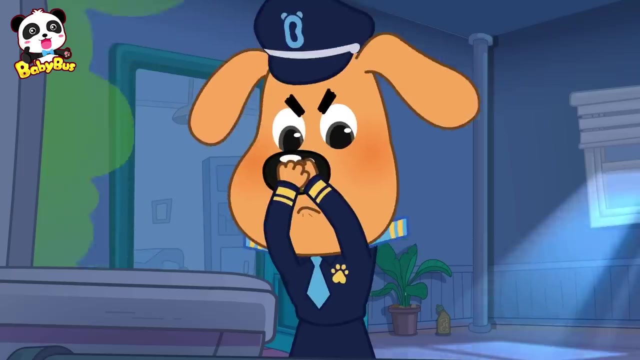 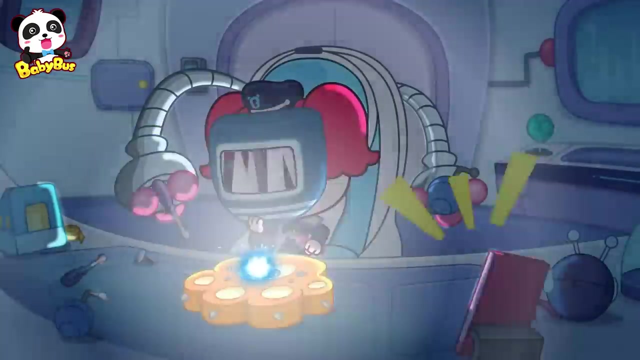 Let's get inside. Hmm, Over there It's coming from here And here, Huh Is the sound moving? Ha, I found it. What's that smell? Huh, Sounds like it's coming from the pipes. Huh, 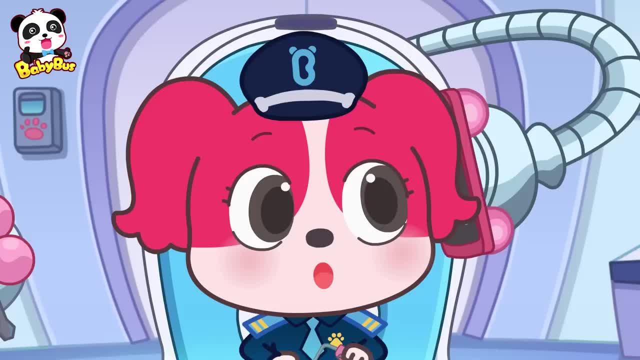 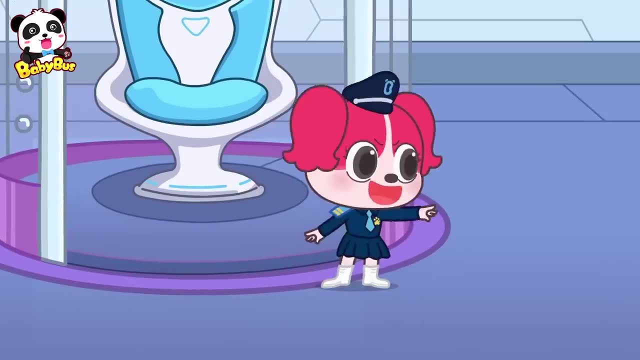 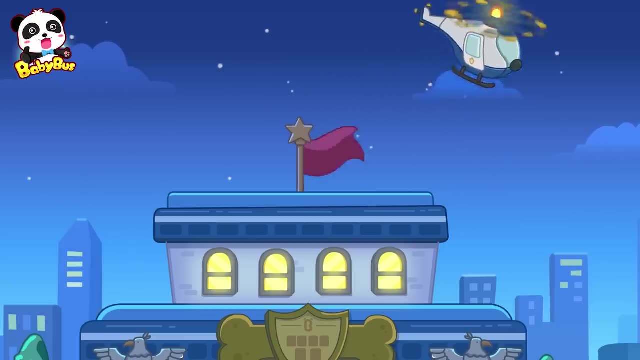 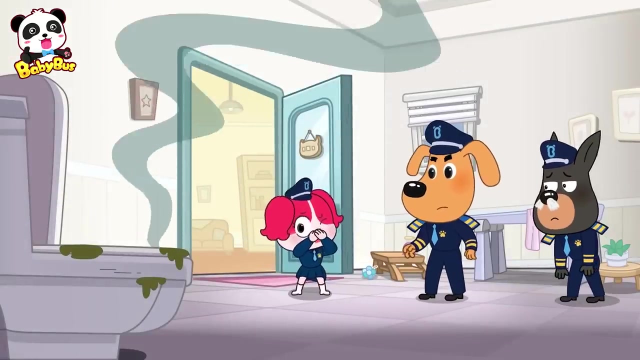 Woof, This is Papillon. Papillon, we need your backup. Got it? Yes, Papillon always has a way. Sheriff Labrador, Uh-oh, How can I help you? There's something in the pipes. Hmm, I need you to search there. 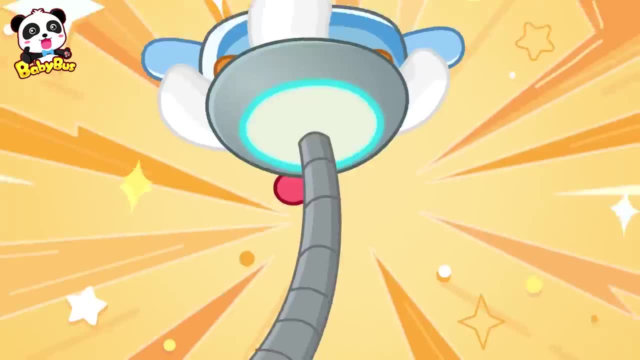 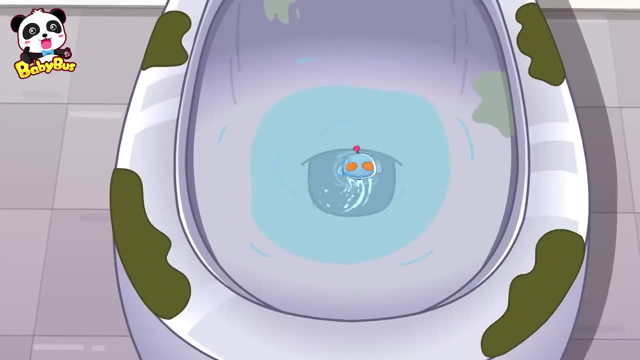 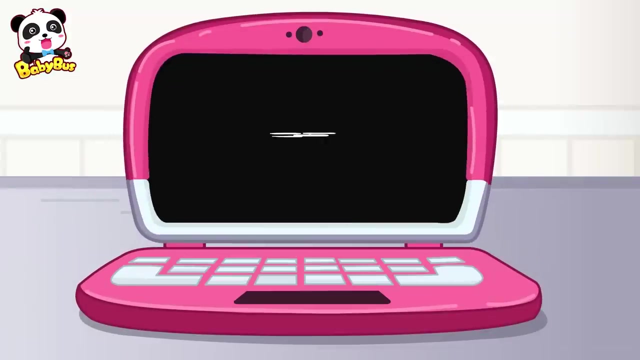 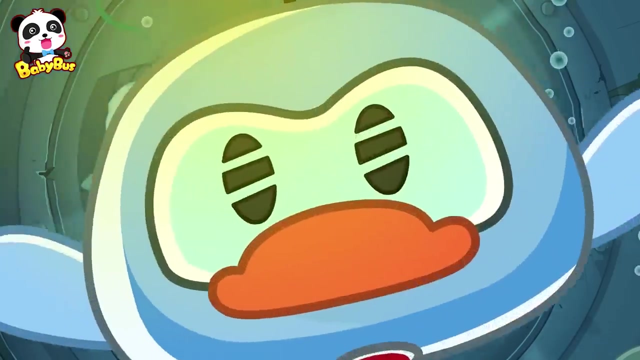 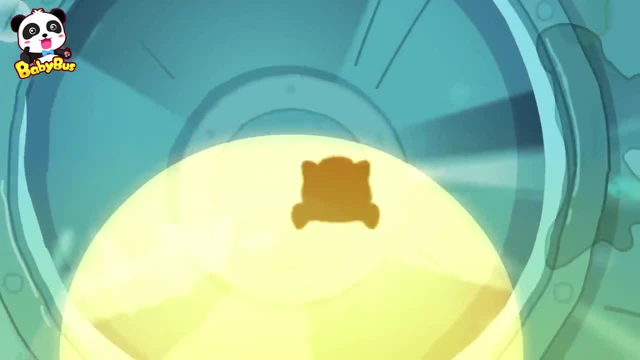 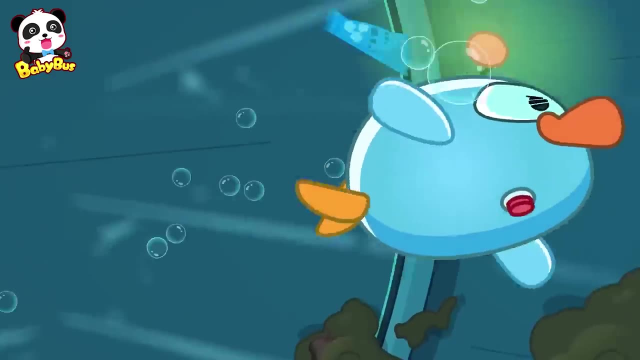 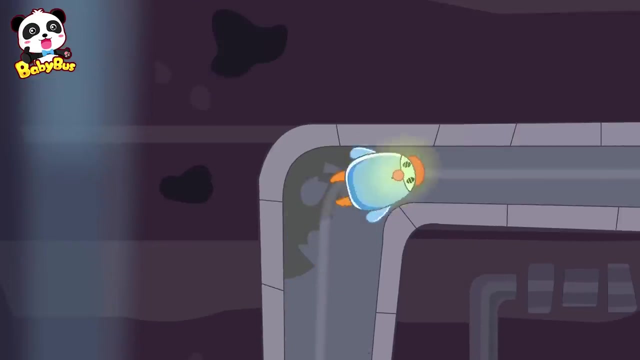 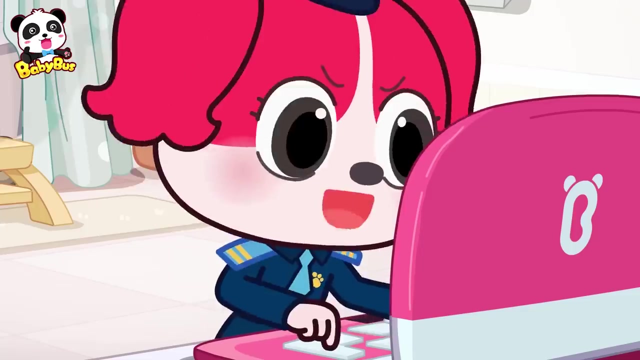 I, I, I, I, I, I. I'm stuck in the pipes. Look something's moving, Follow it. No problem, Come on, come on, I got you, I got you. Clink, Clink, Clink. 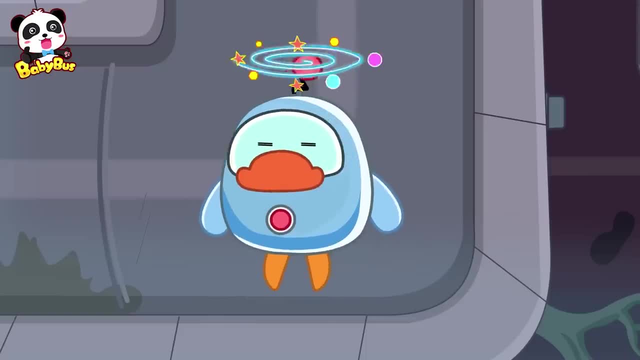 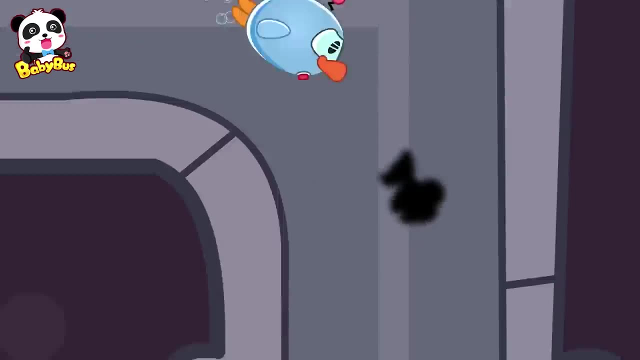 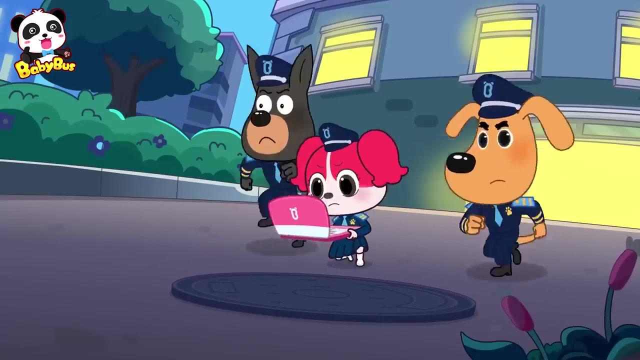 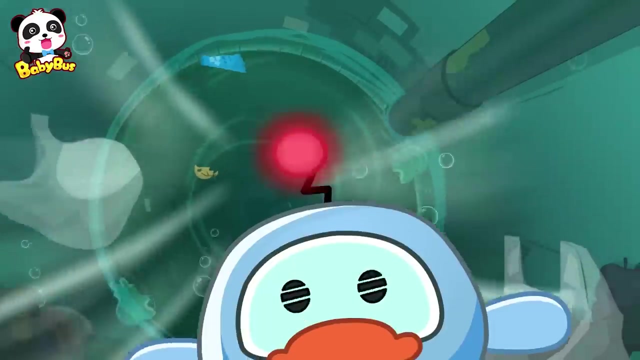 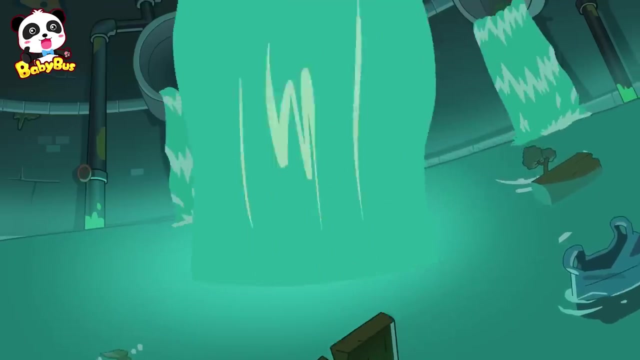 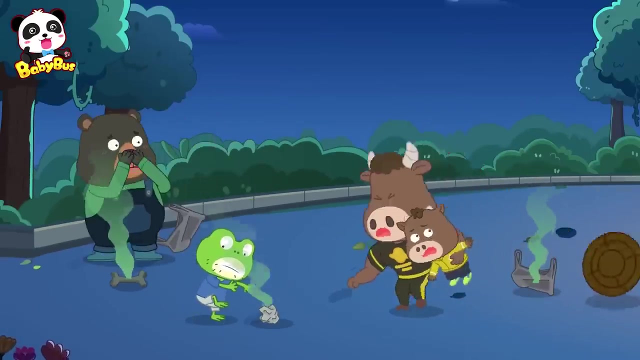 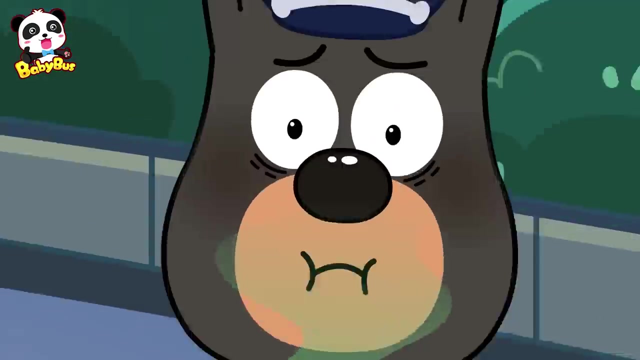 COMPLETE, COMPLETE, er. uh, uh, uh, uh. It went down into the sewer. Let's go downstairs Right now. Little Pepper, It stinks Hey, Hey, Hey, It stinks A fish, It's my fish. 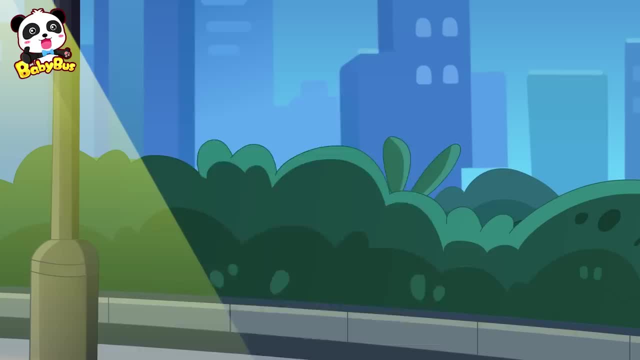 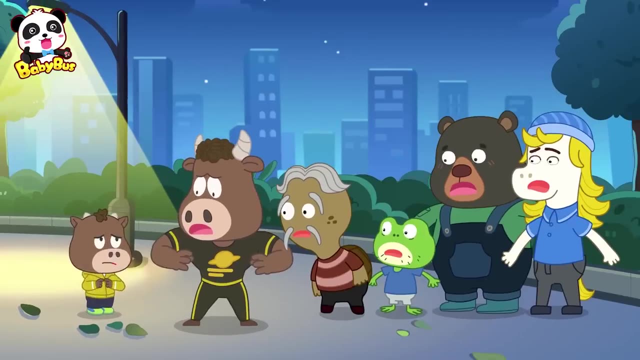 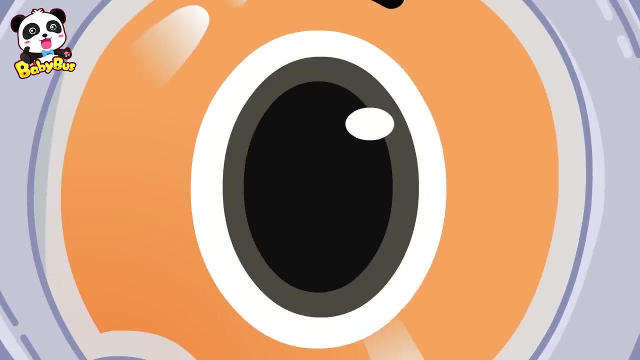 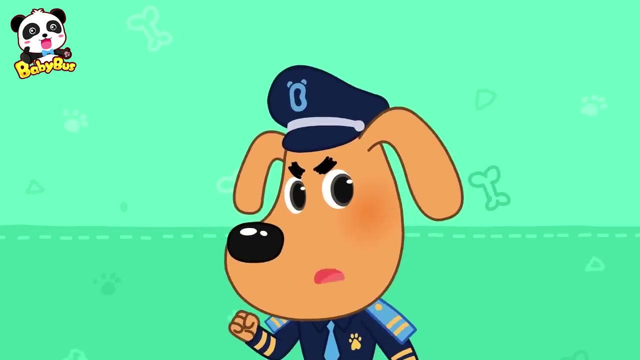 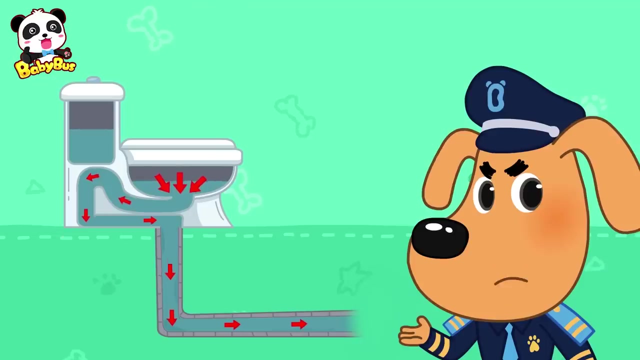 How did it get here? I'm sorry I dropped it in the toilet while playing in the bathroom. Oh my goodness, Sheriff Labrador, Safety Talk Kids. the toilet is not a toy, are connected to sewer pipes and there are a lot of dirty things in the pipes, so don't play. 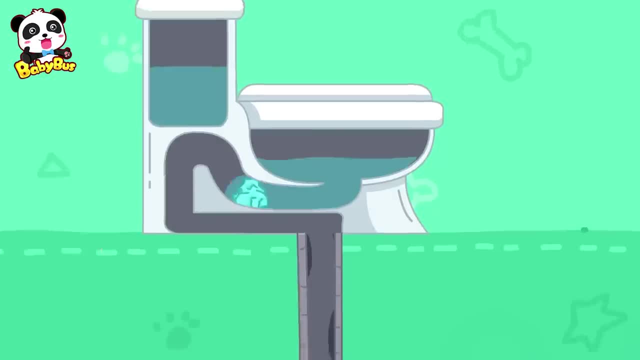 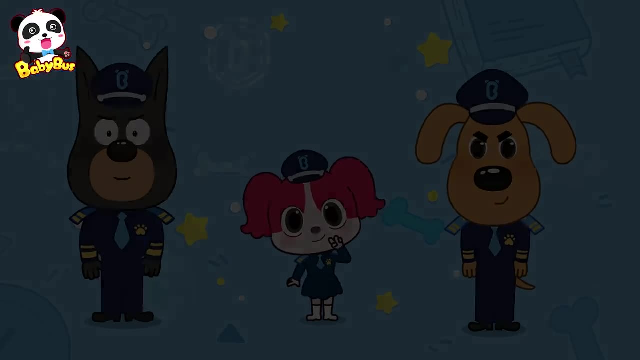 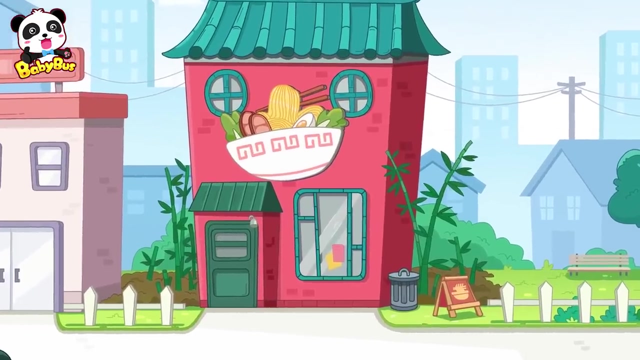 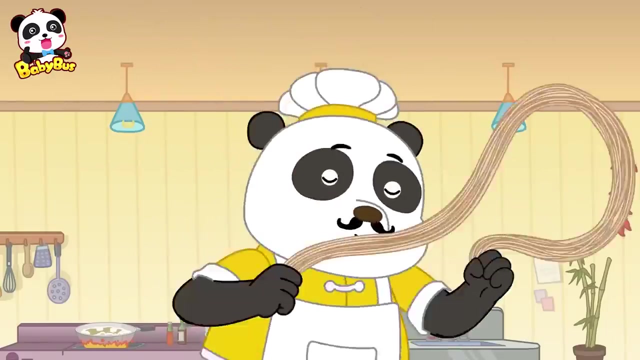 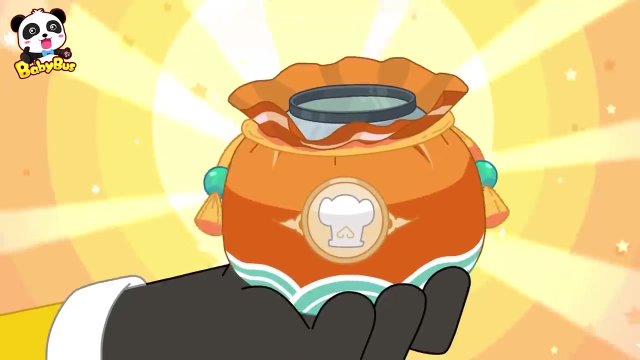 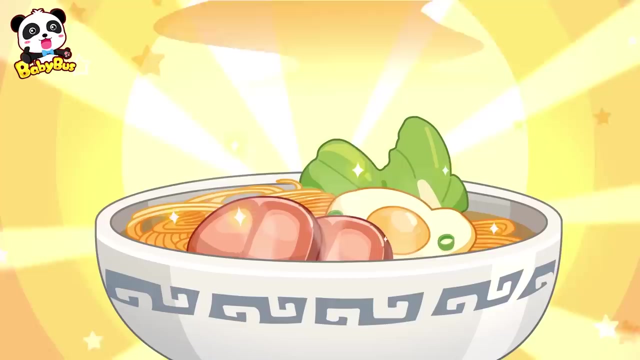 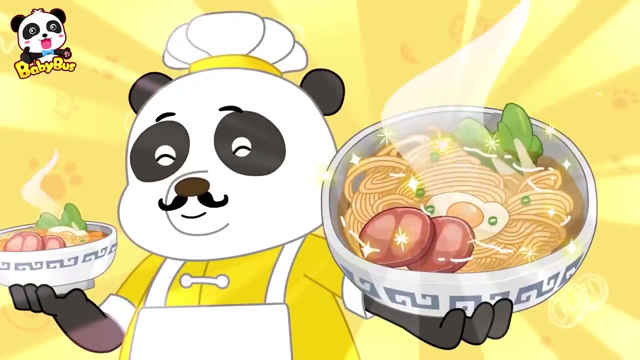 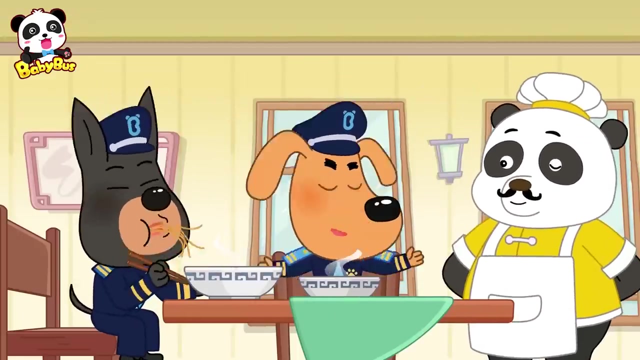 with water in the toilet and don't throw things into it. it'll clog the toilet and cause a big problem. the dangerous kitchen, oh, smells so good. two bowls of our signature noodles. wow, it looks so yummy. mr panda, your noodles are amazing. that's because of our secret spice mix. 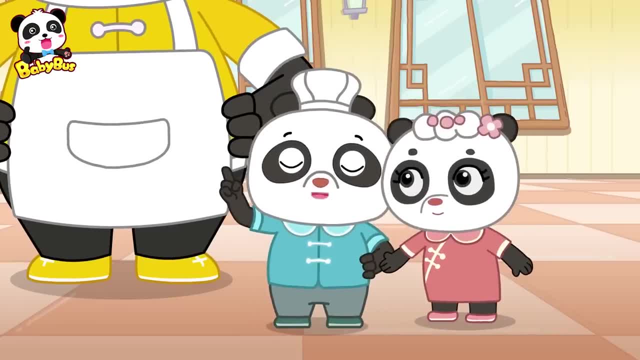 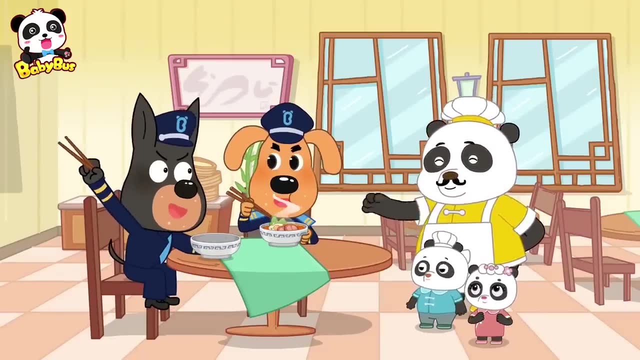 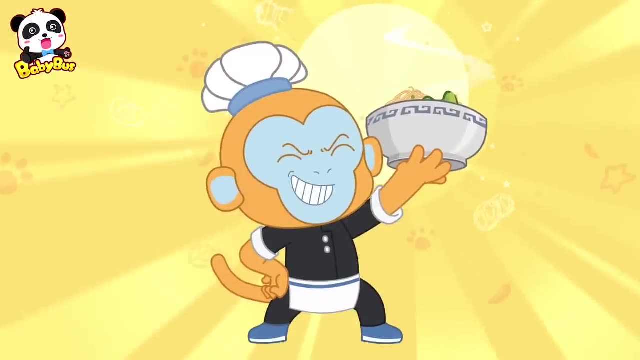 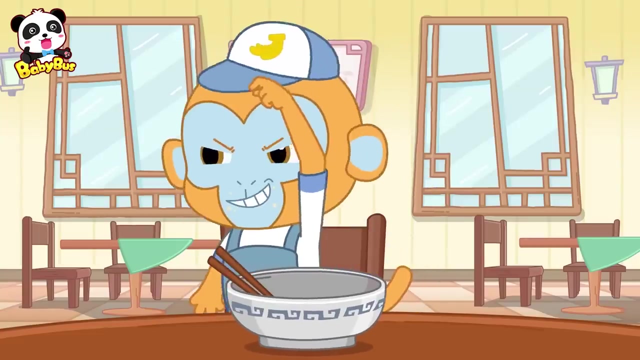 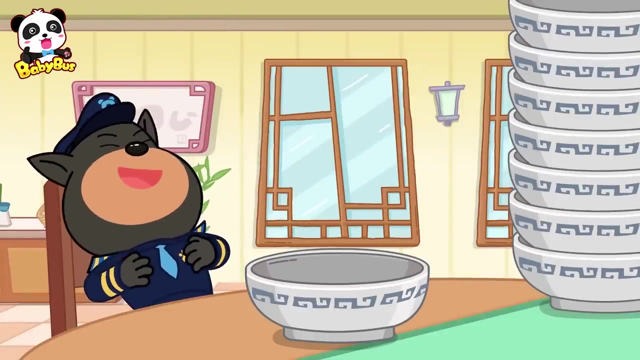 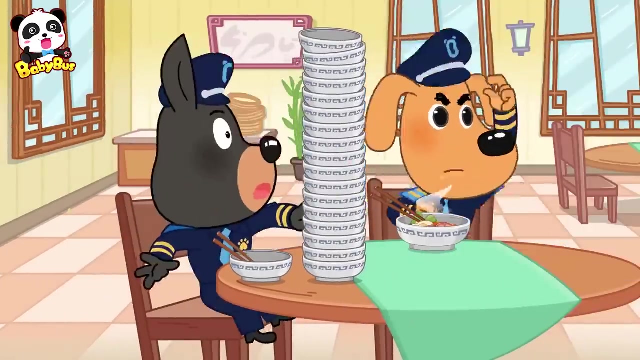 secret spice mix. yeah, the recipe's from our daddy's, daddy's daddy, that's right. oh, another bowl please. if i had the secret spice mix, i'd be able to make yummy noodles too. amazing. another bowl, please, mr panda, what happened? let's go and have a look. 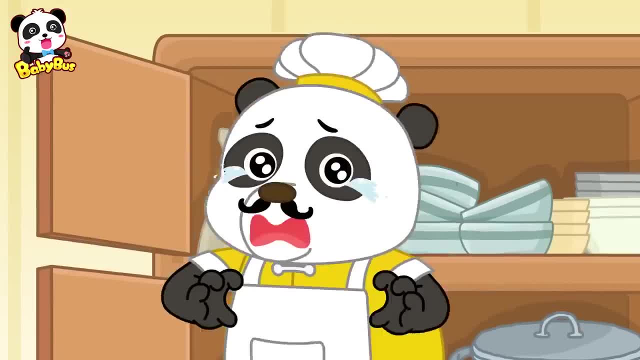 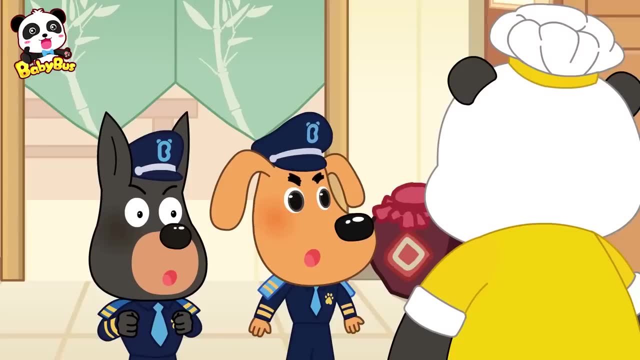 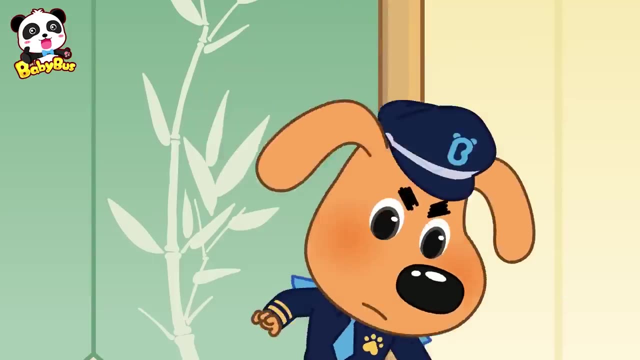 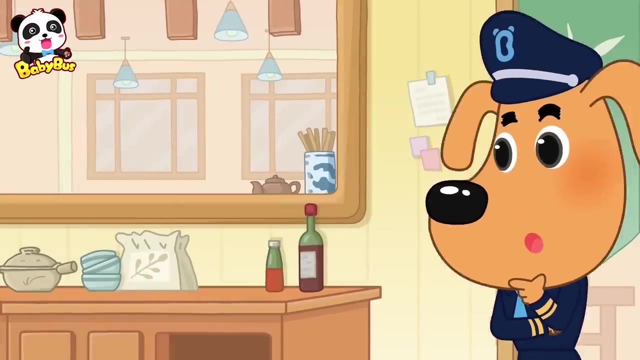 mr panda, what's wrong? sheriff labrador, my secret spice mix is gone. what it's handed down to me by my family and now it's gone. please help me find it. don't worry, there's no case that i can't solve. if it was stolen, there must be clues left around here. dobie, let's split up and look around. 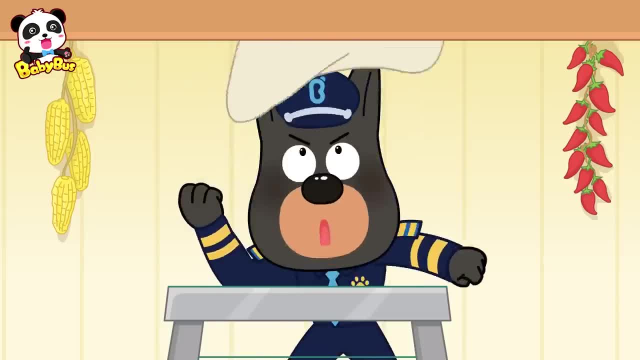 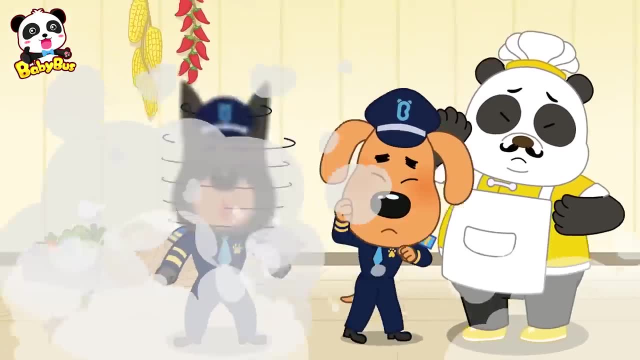 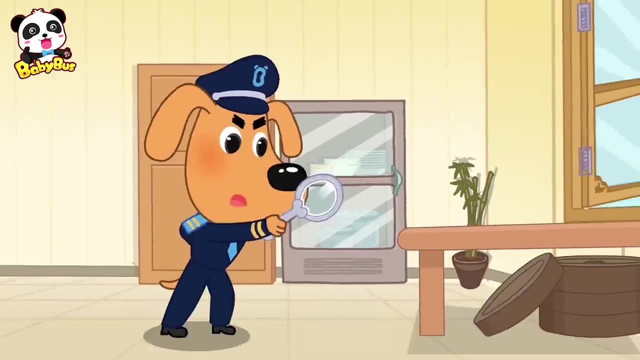 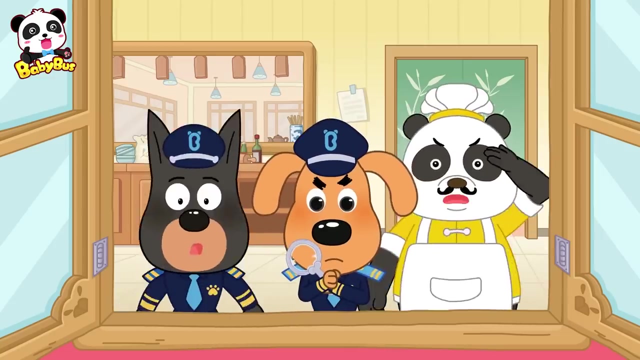 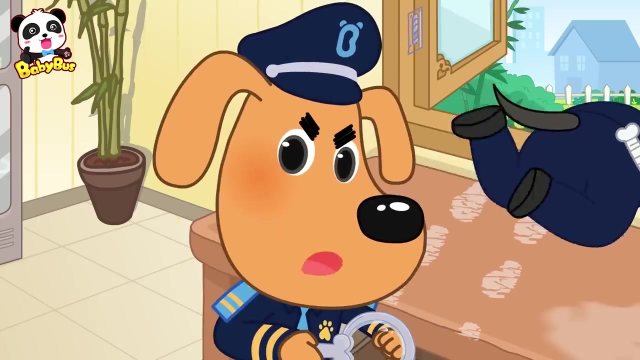 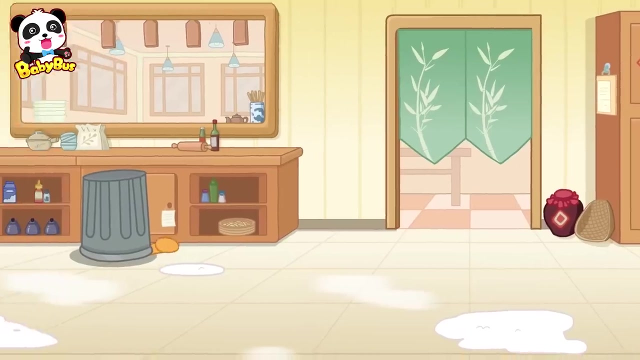 there's the thief. ah, it's just flour. huh, huh footprints. it looks like the thief broke in through the window. huh, unbelievable. i'm gonna catch the thief. the thief might still be here. what look? there are no footprints leading out of here, so the thief must still be here. 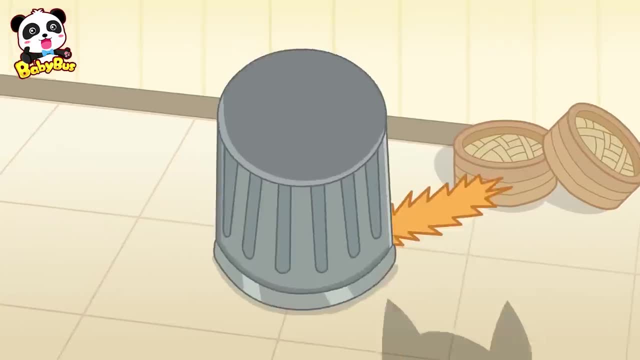 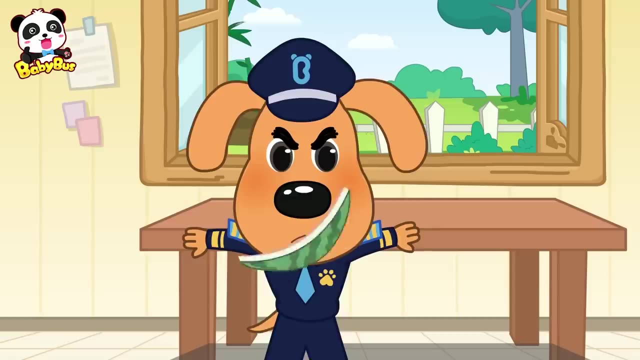 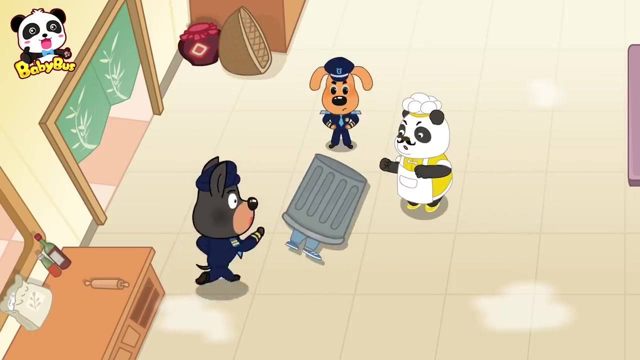 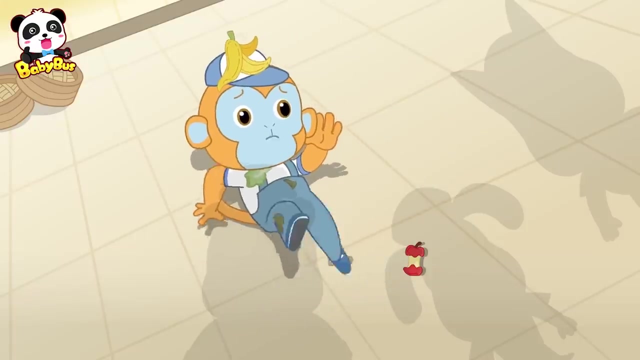 you can't run away. i got you. stop right there. oh, Mr Monkey, it was you. Oh no, it wasn't me. I'm sorry. I just wanted to see how the noodles are made. I didn't steal your spice mix. 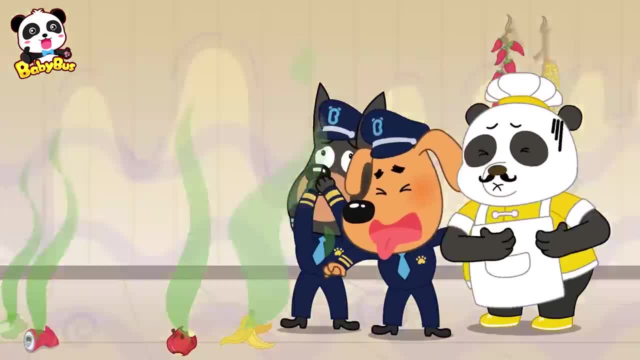 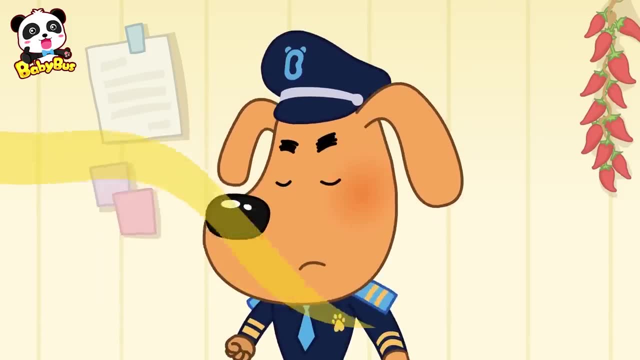 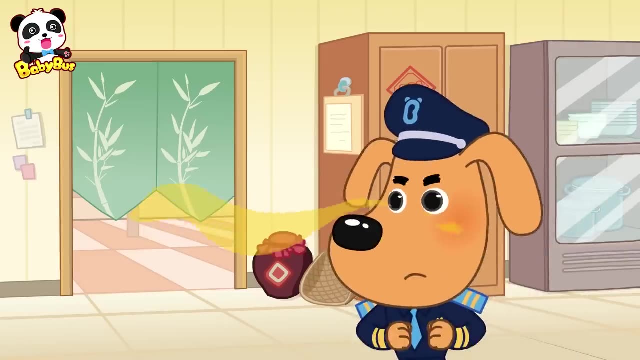 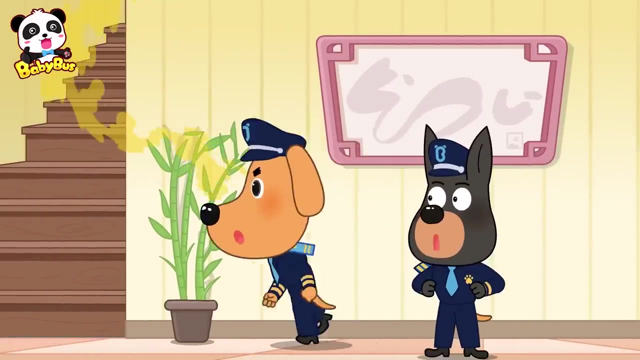 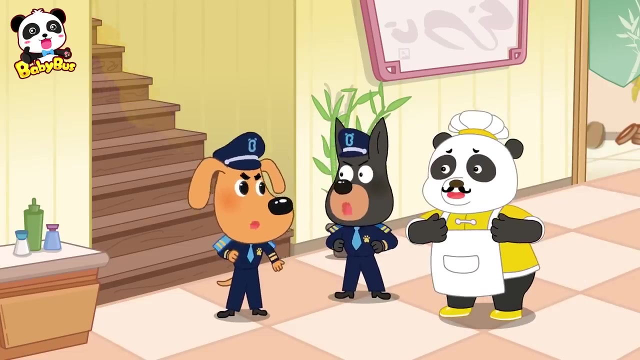 You can search me if you want. If it wasn't Mr Monkey, then who was it? I think I smell the spice mix. Follow me, The smell's coming from up there. There's another kitchen upstairs. Come on, let's go.